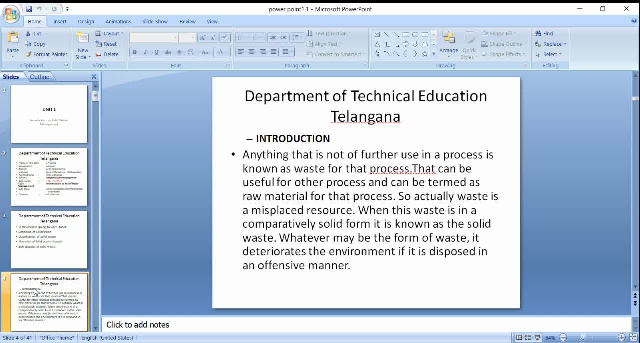 So that it should, it should be useful for further climatic conditions. You can say not affected to the environment, like that, should use the raw materials. So anything that is not for the use in the process, Generally it is not as a waste So that raw material should be in the process or it should be misplaced resource. so that the waste is in a comparatively solid form. it is known as a solid waste. 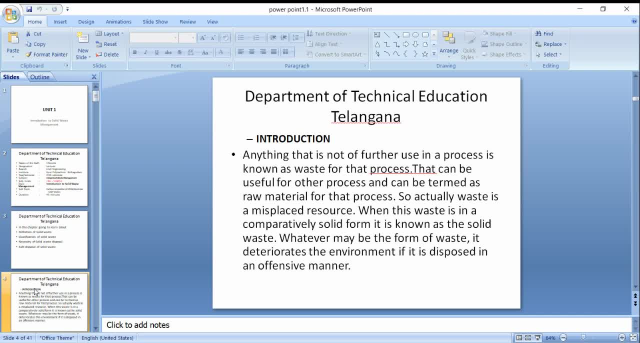 So the waste which is a raw material which is not used should be in the solid form so that it is called as a solid waste. So whatever be the form of a waste, it will cause environmental pollution. So if it is disposed directly it will give offensive smell. 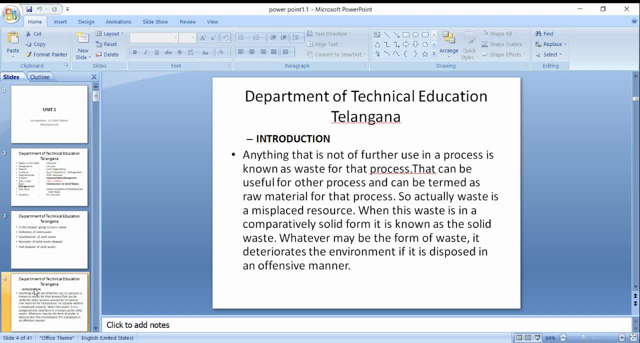 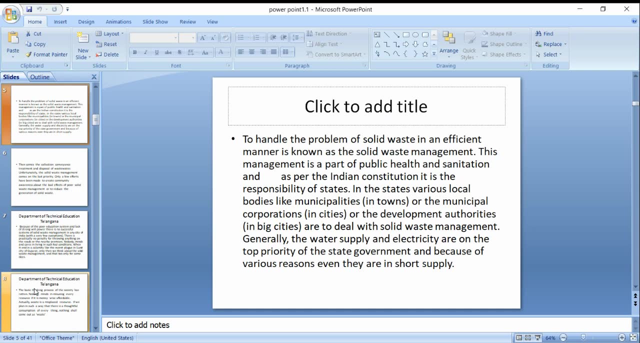 So to control those solid waste problems should be efficient in efficient manner. so there it forms a solid waste management. So it's solid waste management very important. So where it comes, the waste, the solid waste which is not directly put it on, directly put it into the environment. so to control that waste management has scale. 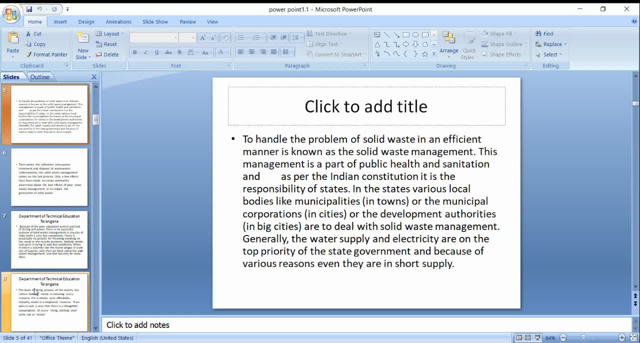 So this management is a part of public health and the sanitation, so it is a part of the public health and sanitation. So our Indian constitution is the responsibility of different states. We have different states, so they will the municipalities in the differences. they have different municipalities, so the municipality will look after those solid waste. 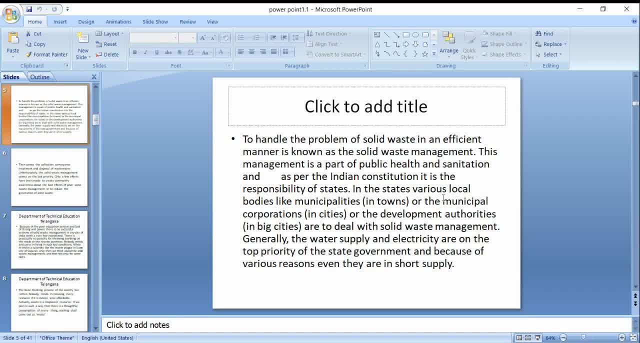 So in the states various local bodies like municipalities are. the municipal corporations are there, So they are. the development authorities are to deal with the solid waste management. So the solid waste management which is directly deal with the municipalities. So generally The water supply and electricity are on the top priority of the state government. 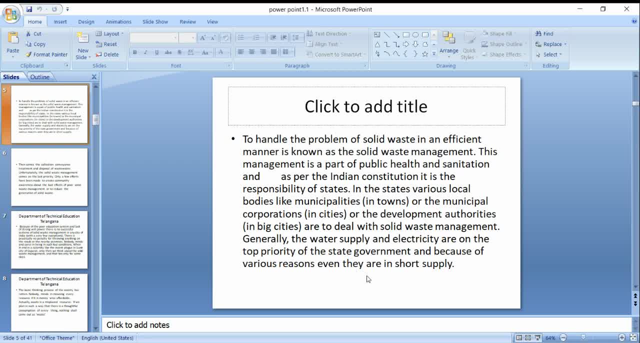 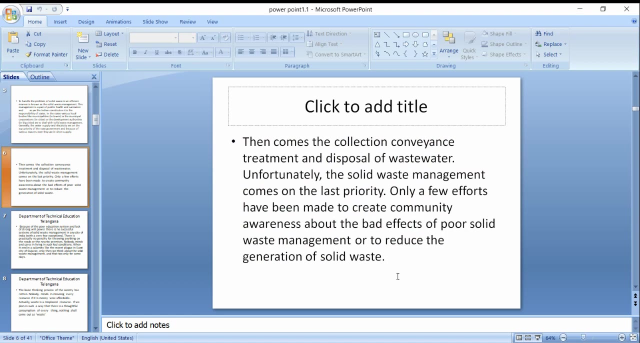 Because it's a various reasons, even they are in short supply. So water is most important. at the same time, this electricity is also important, As in death. equally, now it is waste management is also becoming, because it is also creating the environmental pollution, Also creating the environmental pollution. 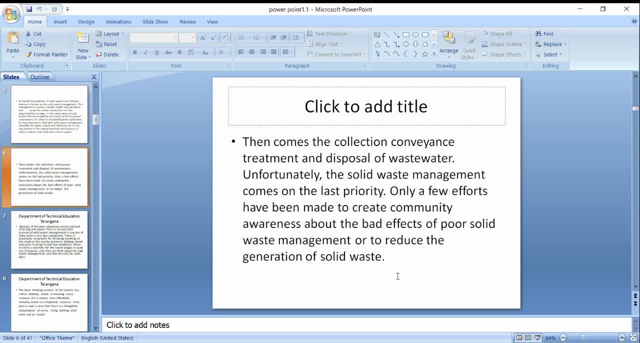 So that then comes the collection, double waste, How you have to collect the waste management and how we have to treat that one and how we have to dispose that well, So there are, unfortunately, that's already. the waste management comes to the wastewater that will be connected in the sanitation or can safe from the Duty household's kitchen. 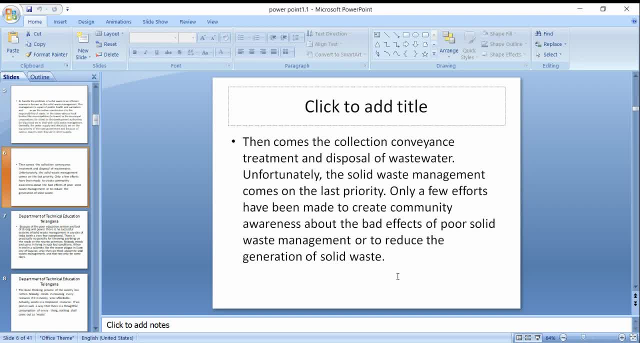 So there are, unfortunately, that solid waste management comes to the waste water that will be connected in the sanitation. All right, you can see from the Household kitchen. All right, the water which is coming from the bathroom. Everything get clean, but it becomes a yesterday. 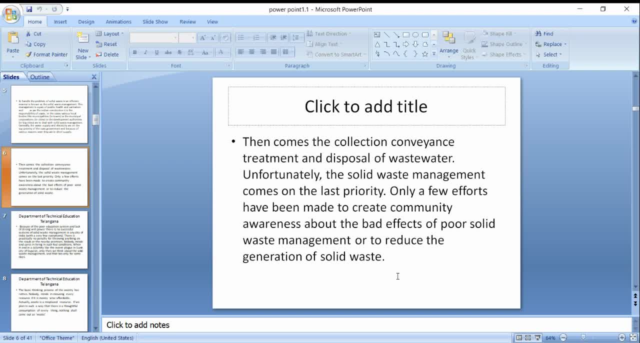 After that are correct, collected into the drains and that will come into an into drain water. but the solid fields will not be collected. there should be collector, some deba, some management should be there, so those, the municipality, will collect those solid waste. so only a few efforts have. 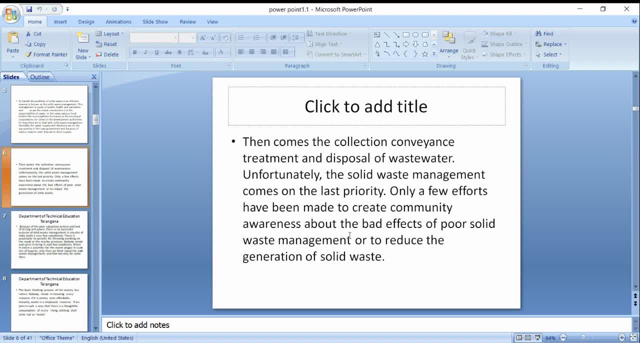 been made to create a community. so awareness about the bad effects of the poor solid waste management are to reduce the generation of the solid. so if we give awareness how it will come affect the environment, then the solid waste can be reduced by storage and by throwing out in a systematic way. so if you've thrown it directly, uh, to those. 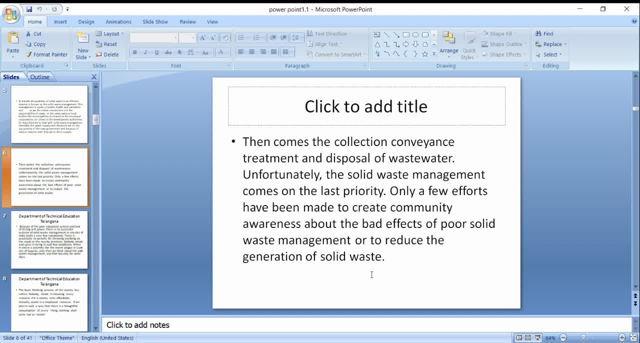 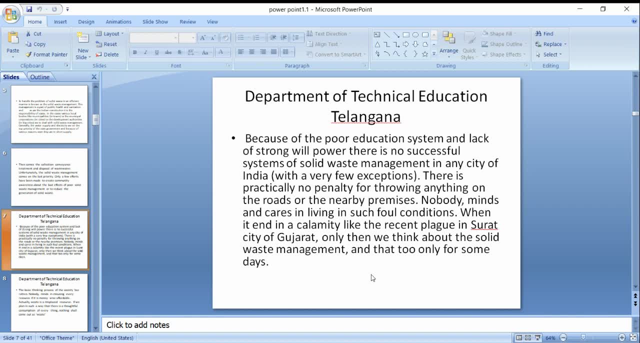 open dump yards, then it will create a environment pollution, so that should be given. so because of the poor education system and lack of strong willpower, there is no successful systems of solid waste also. solid waste management is also present. is is a powerful tool. become no successful systems. no one is giving importance to that one. so there is a practically 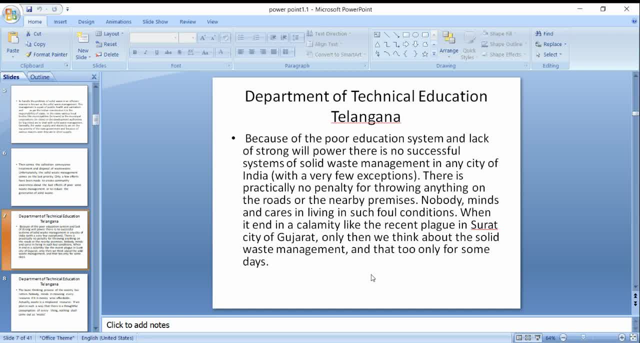 no penalty for them. so if we keep penalty, if you throw the dust outside, if you throw the garbage outside, if we keep some penalty, so the the people will get awareness and they will throw it also. for example, if we go for other countries, then they will put in the separate disturbance. not you can say: 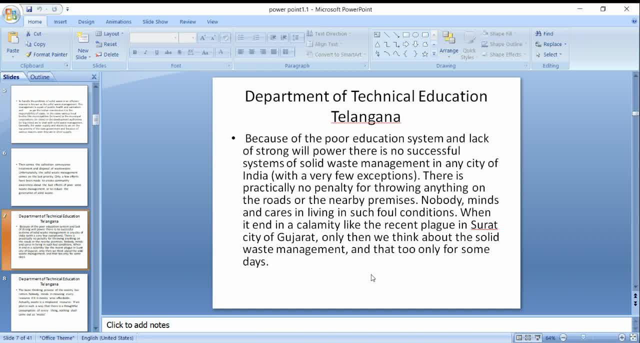 it's a container they will not throw outside on the roads. but in india we will not follow those instructions. so there should be some penalty so that they will get the awareness of this. nobody minds and cares in the living such a fall conditions, so when it end any 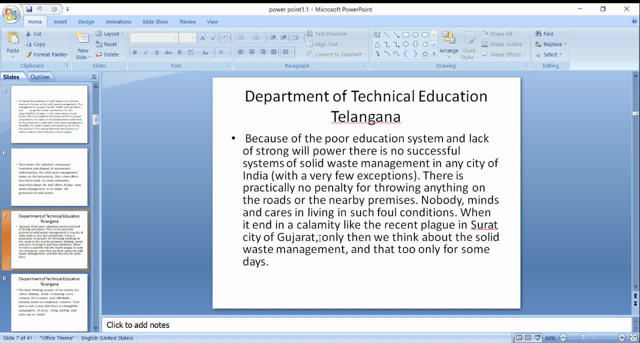 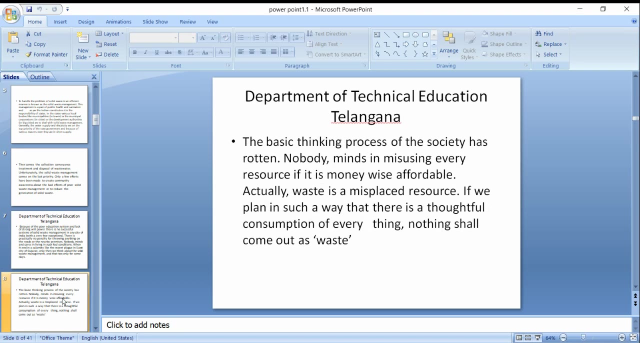 climatic like the. so in the surat and the gujarat there was a disease called plagium that was by the rats. so this this is somewhat uh the rats came due to about the vast solid waste. so for that we have to give the awareness for those things the basic thinking process of the society has. 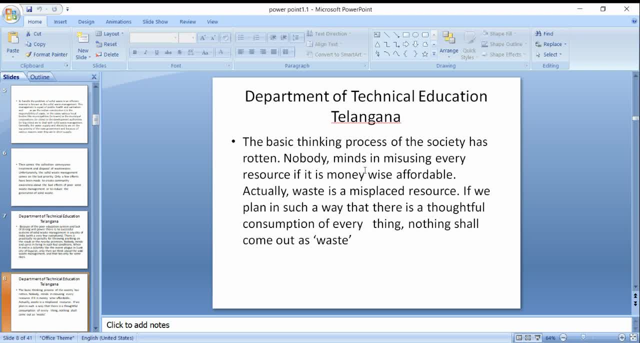 broken. so nobody minds in misusing every resource if it is, in money wise, affordable. so all are thinking um about how we will get it and how money like that, but no one is caring about the pollution, how much we are making the polluted the uh surroundings and no one is care taking care of. so if we plan in such a manner that there 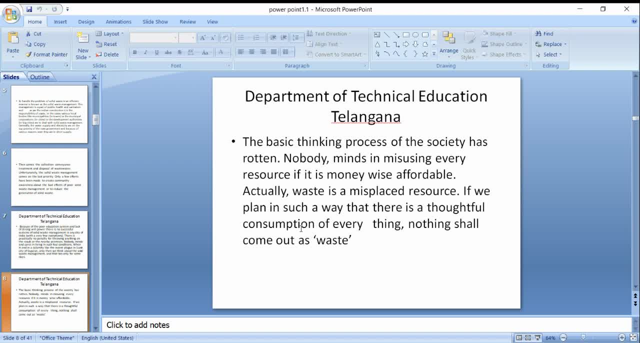 is a thoughtful conception of everything. nothing shall come out as a waste. so we should plan that every way should be recyclable like that. if we plan, then that waste will be uh, useful, uh in a such a way that it can be reused like that, so it will not polluted. 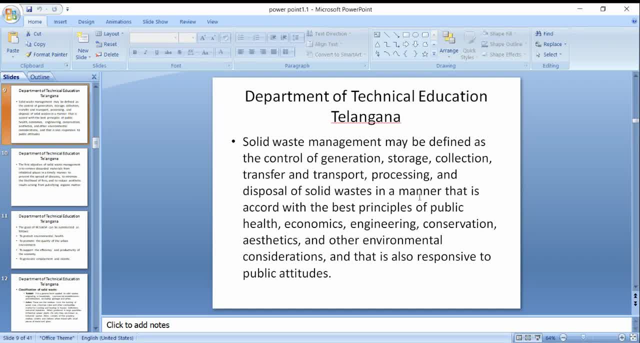 so solid waste management may be defined. what it means it is the control of generation: storage, collection, transfer and transport, processing and disposal of solid waste. so what? it is the uh control of generation. so if we uh, if you use the uh generation, the solid waste should not be more, if we should be uh in the control manner. 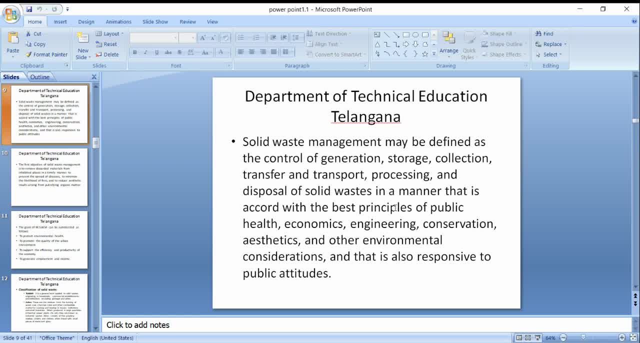 so control of generation, and after getting the waste it should be storage and that storage should be collected and it should be transport and it should be processed, treatment, treated, and after that disposal should be done. so in such a manner is called is an solid waste management. so solid waste management: the municipalities look after the gender. 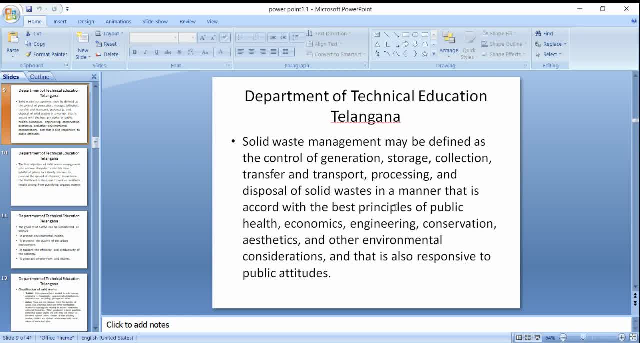 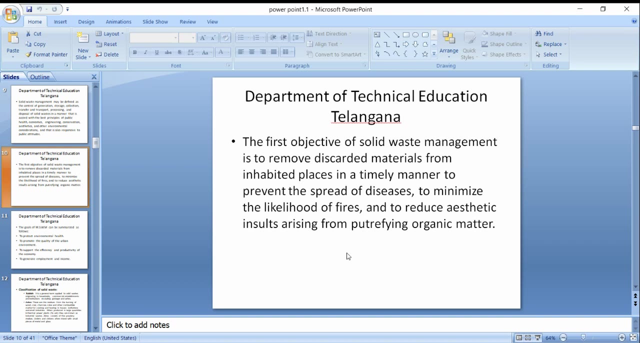 the storage, collection, transport and the processing also. so the best principle of public health, public health departments, economics, engineers, conservations and other environmental countries considerations, so all these other will look after this. the first objective of the solid waste management is to remove the discarded materials from inhabited places in a timely manner to prevent the spread of. 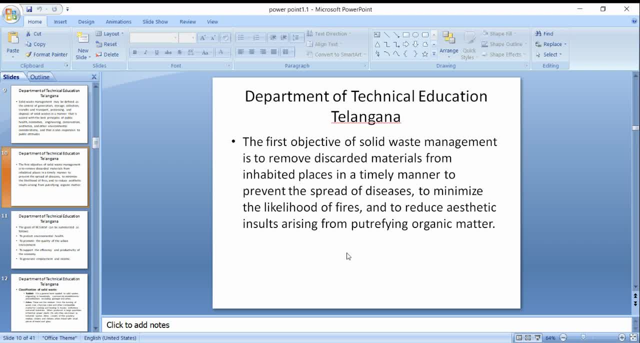 diseases. so the solid waste cannot be keeping for many days, so should be discarded. the material should be discarded timely manner and if so, that it prevents the spread of diseases and to minimize the likely wood of fires and to reduce the ascetic thing in those arising from putrefying organic matter, if you keep like that, the 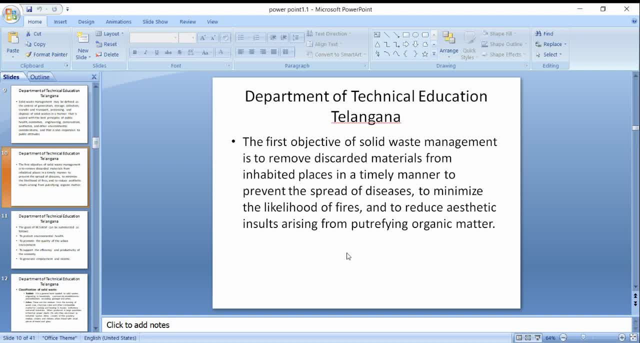 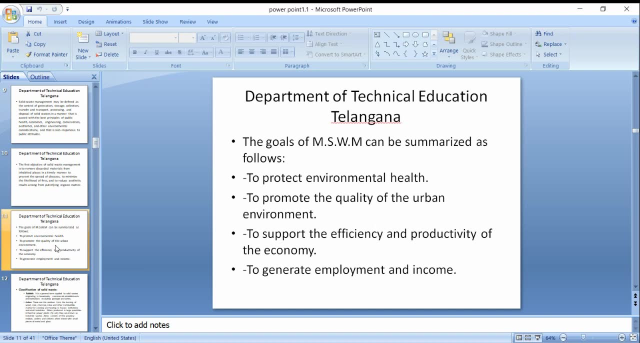 materials will get putrefied and will create a bad smell like that and decomposes them. so it should be thoroughly disposed or discarded from that place. so the main objective or the main goals of the municipality solid waste is nothing but to protect the environmental and to protect the quality of the urban environment and to promote the quality. 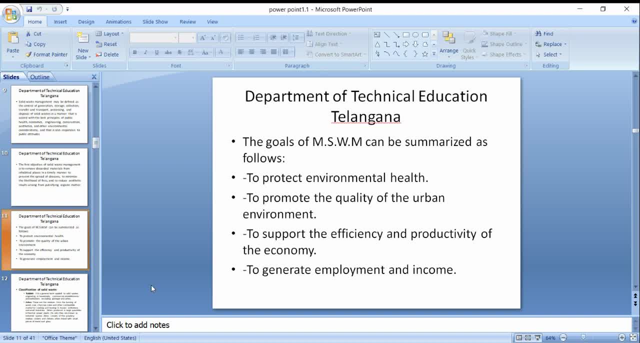 so they will. they have to promote the quality also and to support the efficiency and productivity of the economic and to generate the employment and income. so how they will affect to the income. if the high standard people and the low standard people, middle standard people, are the different incomes are there so different? uh, localities will generate a different. 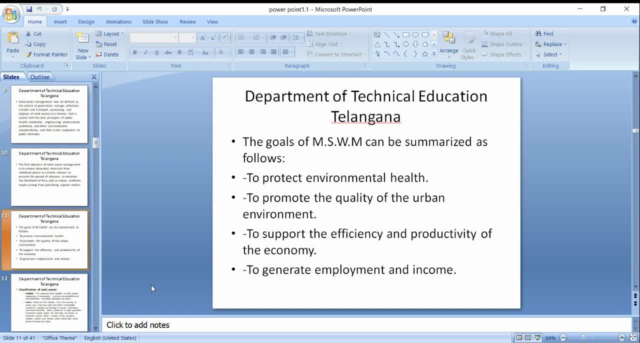 waste. so depends upon their environment, they will generate different types of waste. so those ways should be uh should be taken off to generate further employment also to remove those things we can create the employment also. uh, to take for the municipality uh thing with the employment. for removing the things we can generate the employment and we can if we clean the environment we can. 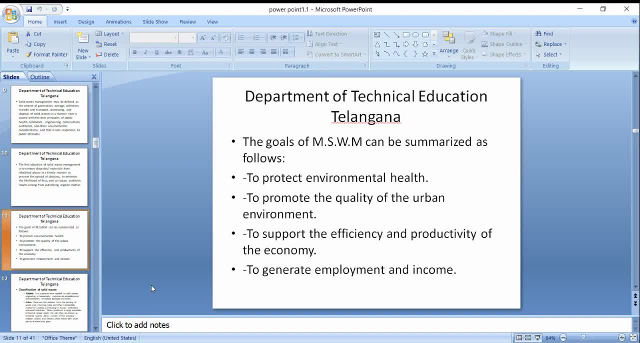 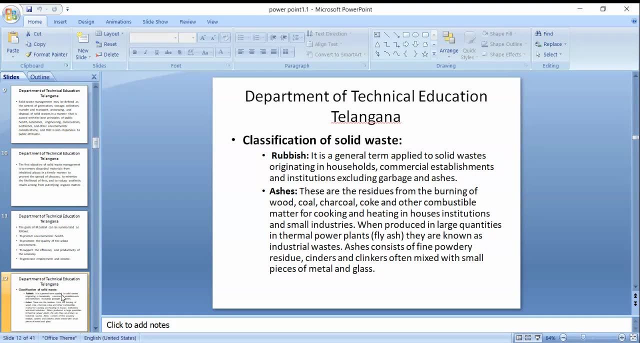 efficiency, productivity also increases. so industrial areas are there if we clean it thoroughly so that we can increase over the economic basis also. next topic is going to classification of the solid phase. so different types are there, so different types of solid. uh ways around 12 classifications are there. so 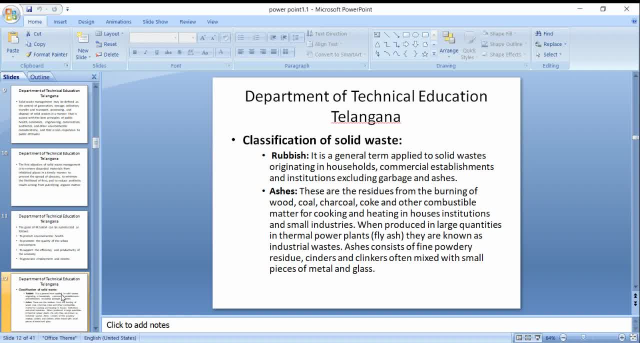 first classification is the rubbish, so it is generally term applied to the solid waste originating in households. so this rubbish will generate from the households a commercial and excluding the garbage and the ash. so garbage means nothing but, uh, in the kitchens, vegetables, vegetable peels or in the kitchen, whatever the necessary things are there, those are considered as a garbage. and in the 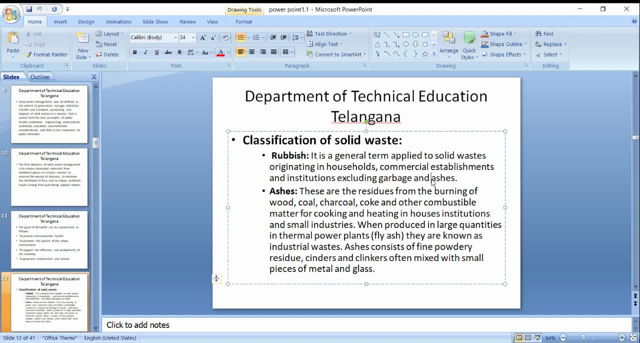 ash. nothing better. the if you use any firing there, the ash will be there, so that there will ash and the garbage is considered as a rubbish. so generally households, uh, and the commercial establishments will have this rubbish. so ash is nothing but wood. this will come from the mines, you can say, or where the industries are there. 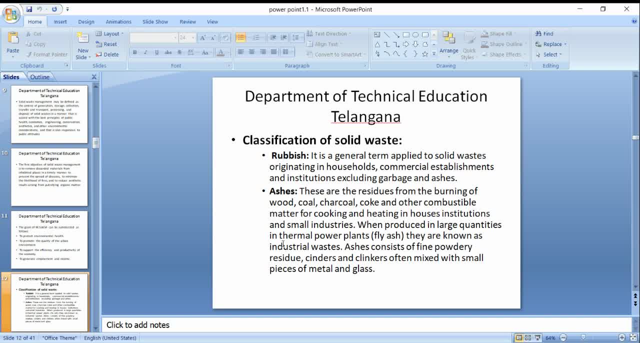 so so come from wood, coal and other composite matter. so for cooking, so ash it's consists of fine powder residue, the cinder sand, so ash it will be useful for the fly ash breaks. also, if we want to recycle it- ash can be used in a correct manner- then it will be useful. if we ure, if we thrown it like that, it will. 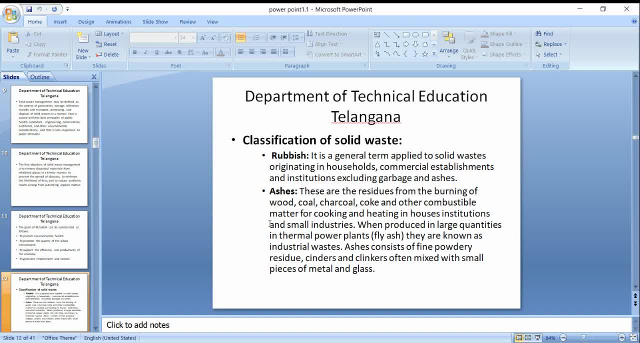 create the dust pollution. so for that we have to see how can be used ash for type of déficit. so we use ash. you can use ash for a lot of matters like garbage, for example cash. how can we reuse reuseful those things so it can be useful for the cement. also we can use in the 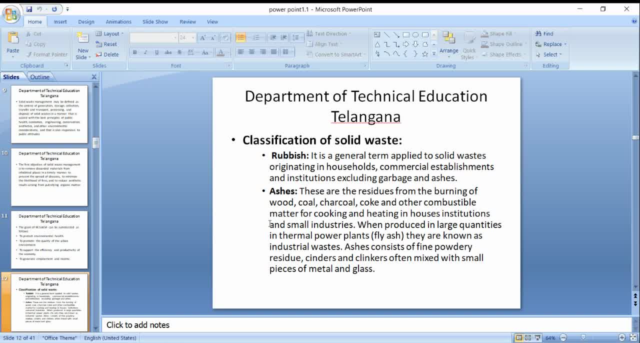 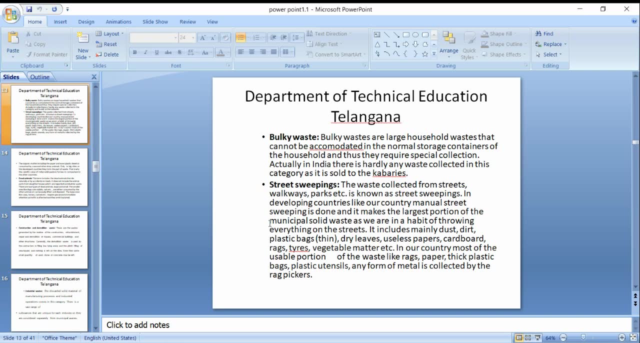 cement for the cement refraction. so when it is produced from the thermal power plants it is used for the power generation also, so they are known as the industrial waste. so ash is the fine powder residue. so bulky waste, bulky based are large households. okay, that can be accommodated in. 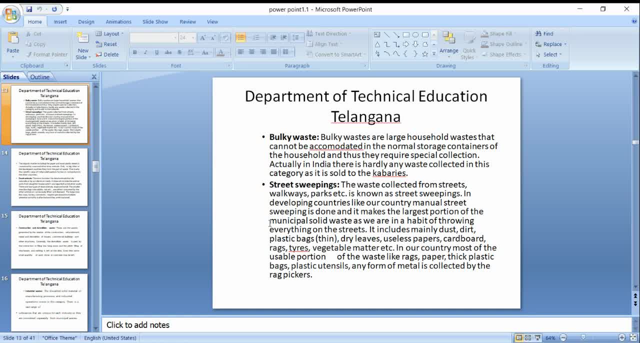 the normal storage containers. so bulky waste is nothing but. four or five families are living together, large waste will become so that should be in stored in the containers so of the household and thus requires special collection. so actually in india there is a hardly any waste collected in the category as it sold to the cabedas. so the waste which was collected 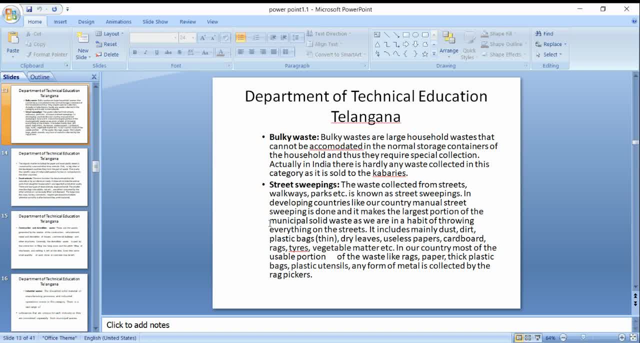 in india. they will be solded and waste plastic or their waste glasses- uh, glass materials are waste, so they will be sold at some places. uh, just like you can say, cabedas, bulky waste will be collected like that. so next comes to street. street sweepings. street sweepings- uh, the 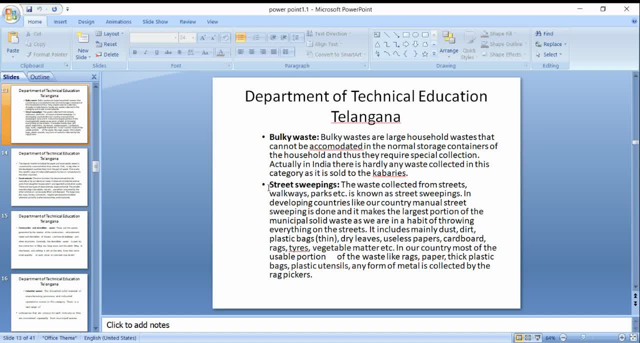 waste collected from the street, so in the streets, where uh the municipalities generally in the morning times they will sweep the streets, so the walk areas and the parks, so that the street sweeping should be, uh collect, uh should be there so that the developing countries like our country, 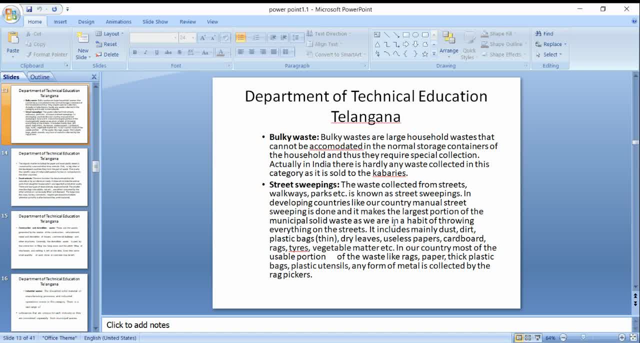 should be there so that if we are collecting the waste, we can collect it there by street sweepings, so that the street sweepings are done and it makes the largest portion of the municipal solid waste, as we are in the habit of throwing everything on the streets, so we will not throw any dust. 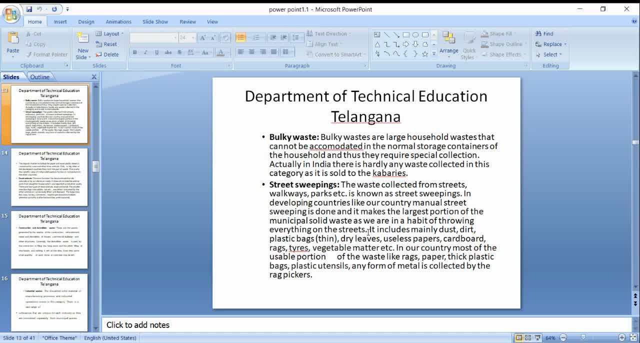 base. so we will throw it as it is. so it should be collected so that the street sweepers are there, so they will remove all those dust and dirt, and major plastic bags will be the dry leaves, useless papers, hoses are generally on the streets, tires, so vegetable mattresses. so in our country most of the 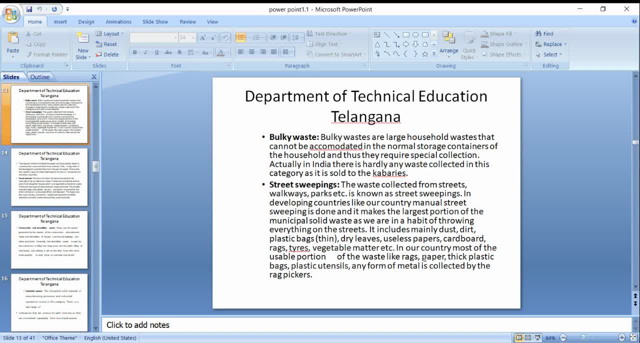 usable portions of the waste, like racks, papers, thick plastic bags, plastic utensils. any form of metal is collected by the rag pickers, so they will collect in a one container just called as a rack. so they will collect. the paper is also recyclable, the plastic also. 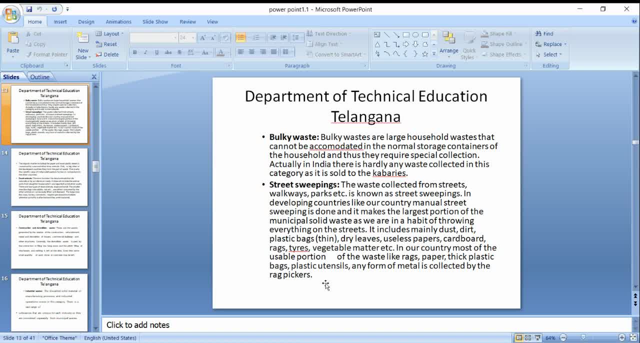 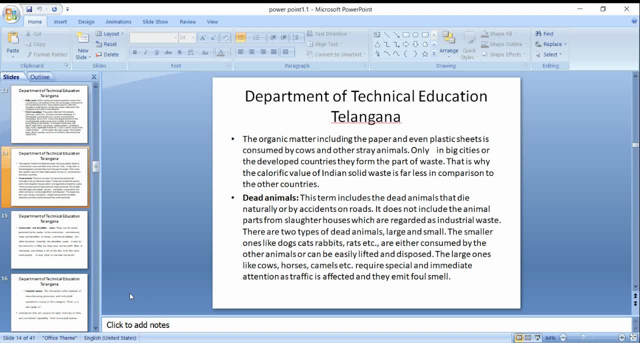 recyclable, so those will be again sent it to the recyclable things. so the tires also recyclable, so those collected and send it to the recycling things. so the organic matter, including the paper and even plastic sheets, is consumed by the cows and others. if you left like that, so they will. 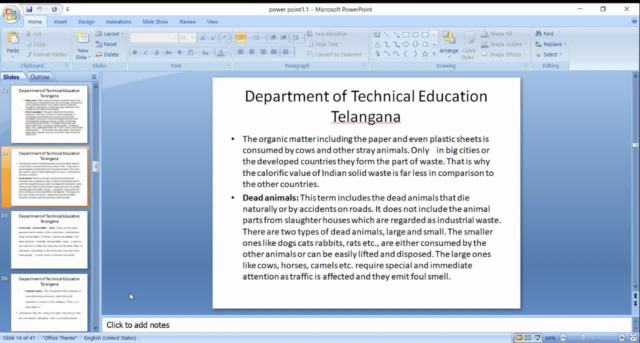 beسمid, and then the waste which is also thats used to collect the plastic also, soall those plastic considered by the other animals which they will get fso, so that will be removed as early as possible. that is the calorific value of india. solid waste is far less and compares to the 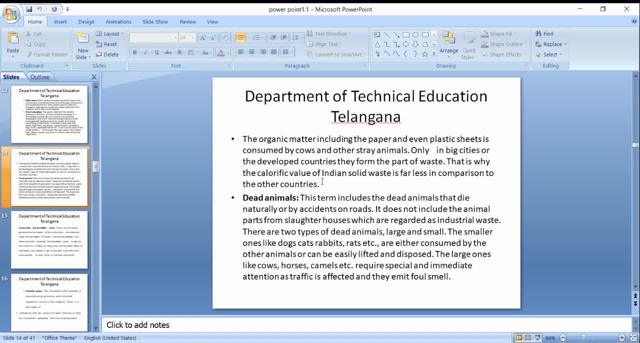 other countries. so the wasted disposals we do. we don't follow the instructions, so we base generation is more comparative to the other countries. so next comes to dead animals. this term includes the dead animals that died naturally are by accident on the roads, so it does not include the animal parts. 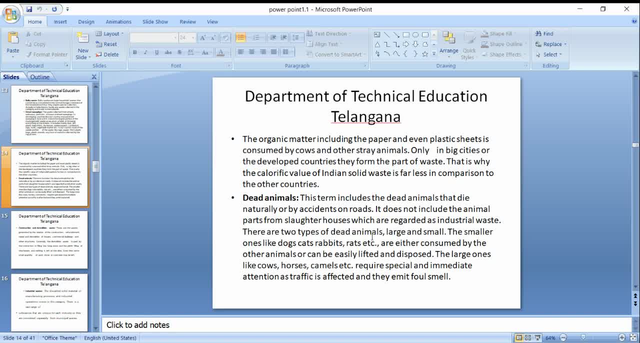 okay and which are regarded as the industrial waste. so these are two types of dead animals, large and small. so the smaller animals are called dog, cats, rabbits, etc. they are consumed by the other animals or can be easily lifted and disposed. the larger ones, cow houses, require special and immediate attention as traffic is affected and they can emit foul. 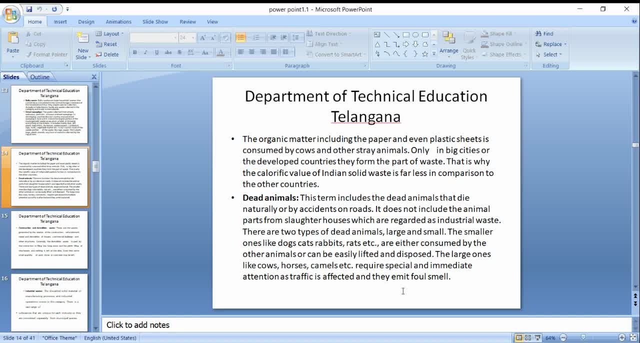 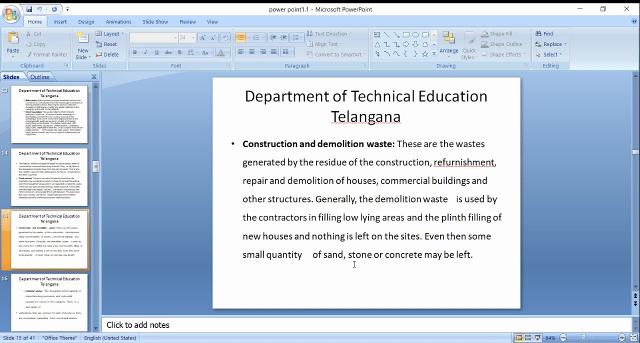 smell. so if we left like that in the areas where they are, the animals are died so it will create the foul smell. so the immediately that was. we uh taken over from that one. so these also cause the environment. next comes to construction and the demolition. construction, construction and the demolition: these are waste generated by the residue. 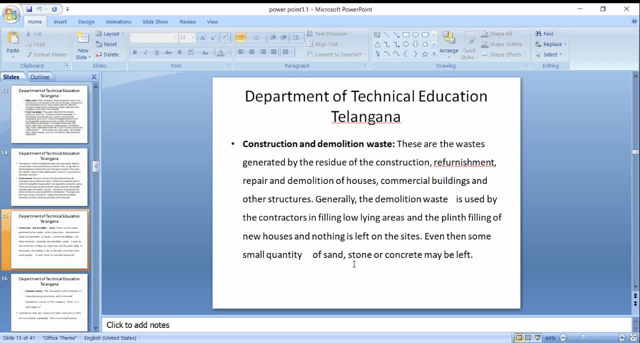 of the construction: refreshment, refurnishment, repair and demolition of purposes. so the based in the generally construction we have the different materials we use. so construction we get the repairs and the demolitions- commercial buildings and other structures. so any demolitions or any repairs are there, the materials will be have to be taken and it 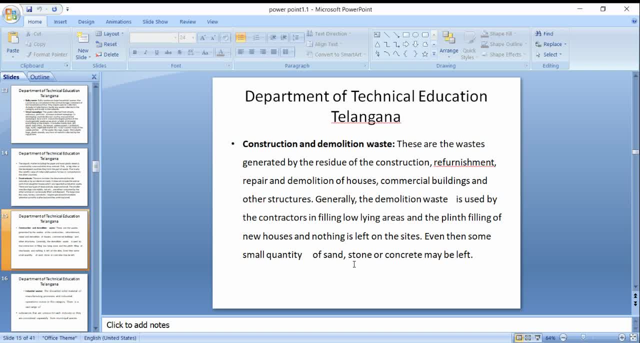 should be reused. generally the demolition waste is used by the contractors in filling of the low-lying areas. so it is rather than the still the concrete should be decomposed are suppressed for low-laying areas till the print filling ends. so if we are constructing the 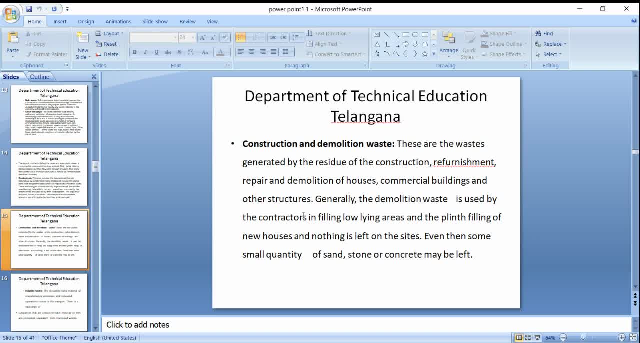 means that uh, demolished material should be destroyed, and so then they are Heh future sweaters. otherwise, also remove wasting with the pier done better or supposed to keep collecting the McC sharpshicke space rather than steel. the concrete should be decomposed, are suppressed for lower laying areas till the print filling aims. so if you are, consideration are new holes that demolishedmented self freeforum use而 cas Hookeriri cookies or easy salary지정iveföruposatuk. 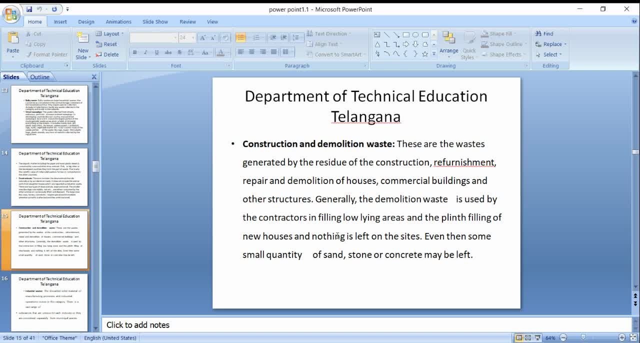 materials are there that can be dumped in the low landing areas and we can increase the height of the plinth. so even then some quantity of sand, stone or concrete may be left. so after, at the time of the construction, we will left some sand and stone like that at the surroundings. we will. 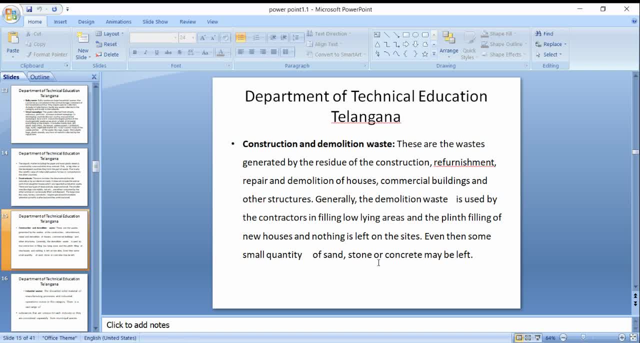 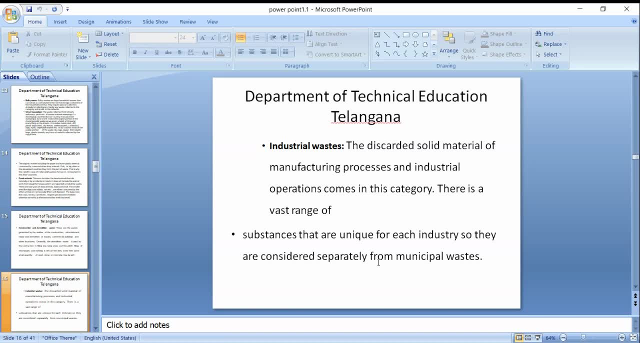 not clean them. so of the sand in the major, the sand will create more pollution compared to the stone them. so next comes to industrial weights, so industrial ways that this discard solid material manufacturing process and industrial operations come in this category. there is a vast range of substance that are unique for each industry, so different industries. 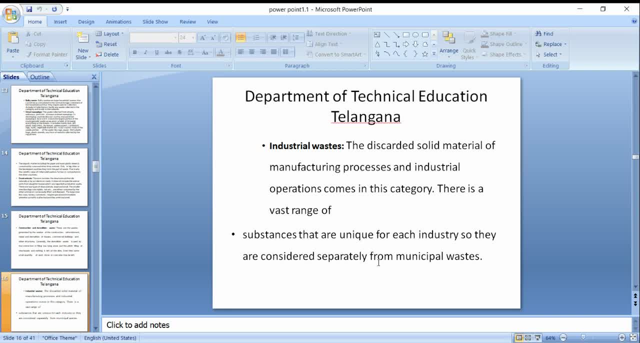 produce different types of waste, whether it must be plastic industry and glass industry, food industries. different types of waste will be manufactured from the different industries, so they should be categorized, and there is a vast range of substance will be good, so that should be for each industry. so they are considered. 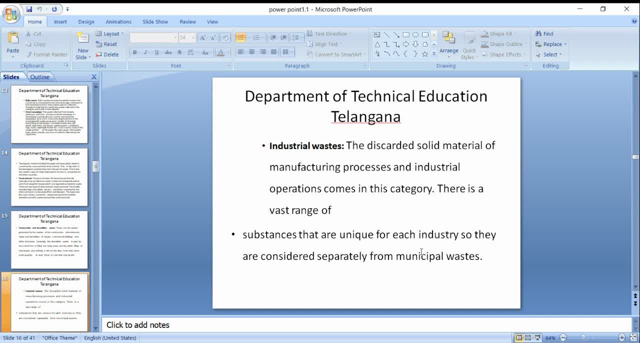 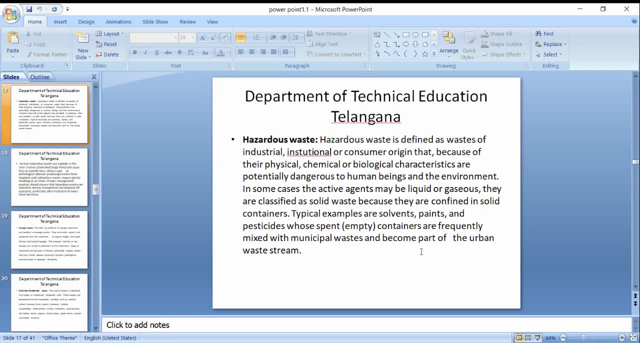 separately for municipal of so from municipal waste, so they are unique and that are connected to the municipal. next comes to hazardous waste. so these are coming from the physical and the chemical properties, as that is means the toxic materials. so there is a coming from the industries. so institutional, consumer origin that. 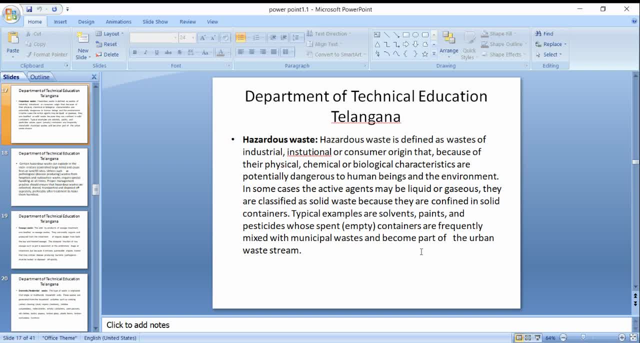 because of the physical and chemical or biological characters are potentially dangerous to human beings. so that if we store the waste for a few days- so it will- the waste will be solid, waste will be get changed. it's a physical and chemical property that is so if the chemical and physical properties have changed, with some 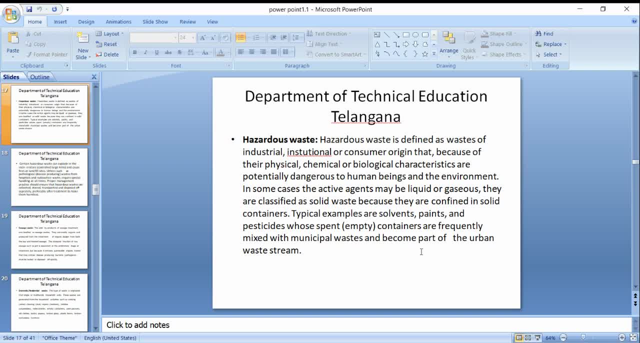 of the materials cause the hazardous. for example, if you left the paint like that, having some chemicals, it will create the hazardous. so in some cases the active agents may be liquid or gaseous. they are classified as solid waste because they are confined in the sort waste. so in some cases the active agents maybe alaus sheet. they are close to us as get your. 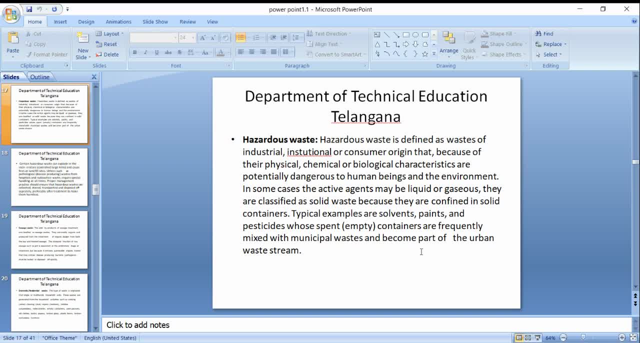 solid waste because they are confined in the solid containers. so solvent paints and pesticides, house spent containers, are frequently mixed with the municipal waste and become part of the urban waste system. so, like that, the poisonous thing you pick, you store for many time. for a time they will. 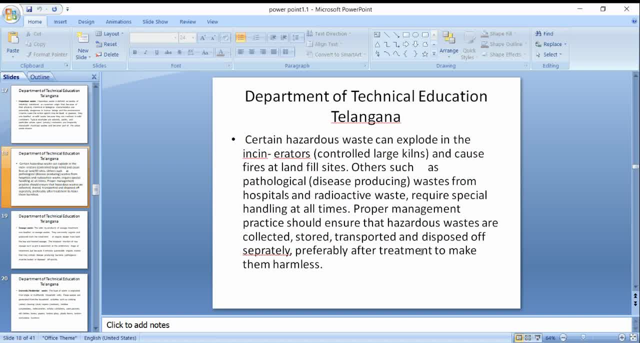 create it. so certain hazardness will. waste can explode in the insulators. so those are to be stored in the controlled large kills. so they should, they will, should not throw it outside. so it should be collected in one container and should be stored in large containers, so in class, so it 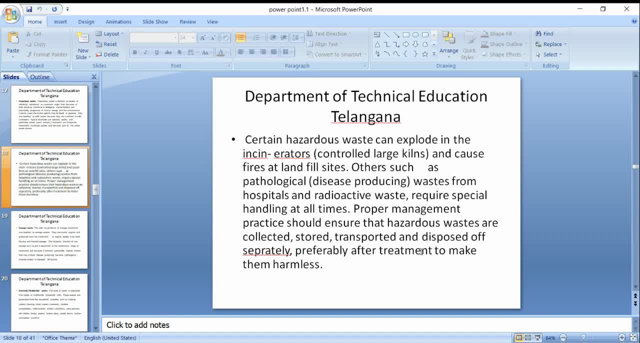 will cause if you not protected. it will cause the fires and also landfills. so such other, such as the pathological, pathological waste from the hospitals and radio waste. so they should also handle the at all times. so proper management should be taken care of this one: collected, stored, transport and disposed of. 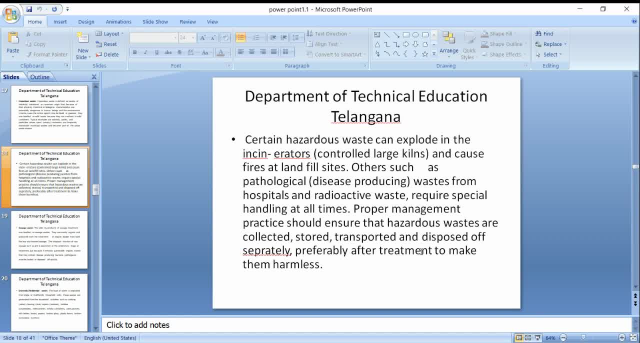 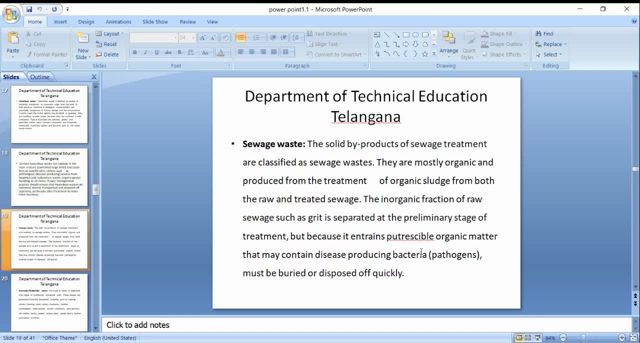 separately, so those should be disposed in a separate containers. so harmful things proxies. so those are. the house that is nice comes to see B the socket by product of 7h treatment and classified as Nou wind solid waste. sewage- sewage waste generally from the bathrooms comes under sewage organic. 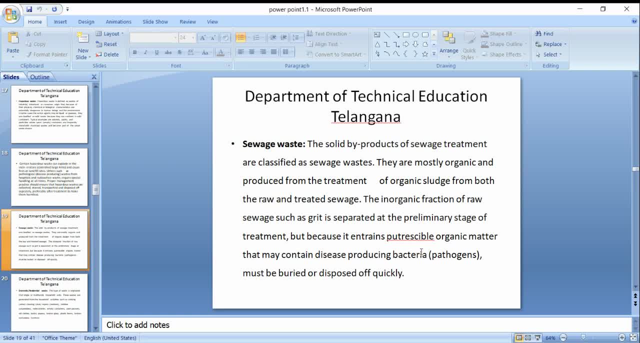 produce that are from the treatment of organic sludge, both raw and treated sewage, so they might be of organic and inorganic fractions, such as grit is separated. so for the sewage they have different treatment plants. we have sedimentation and sedimentation process sludge. 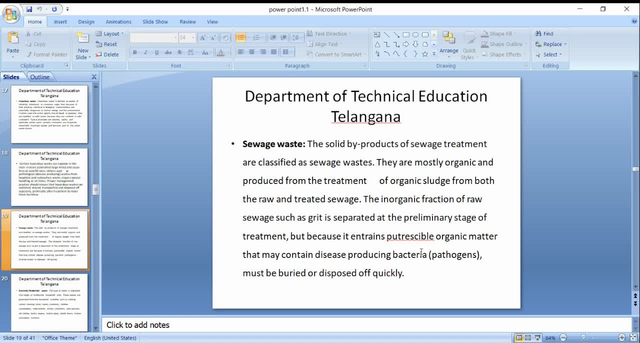 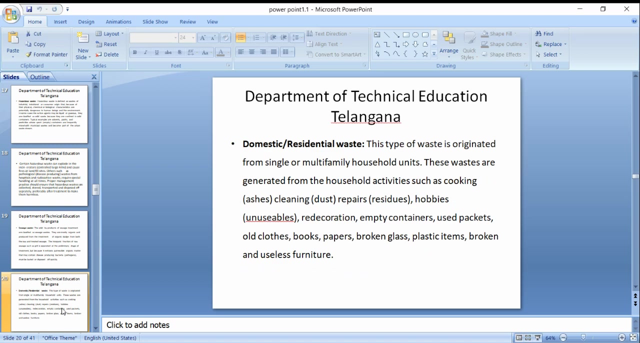 disposals, so different process are there for the disposals and for collecting the sewage. so those because of its entrance artificial organic matter, they may contain diseases producing bacteria, so they should be buried. generally is in 2018, so we will use it- the sanitation septic tanks like that. we will use it domestic. 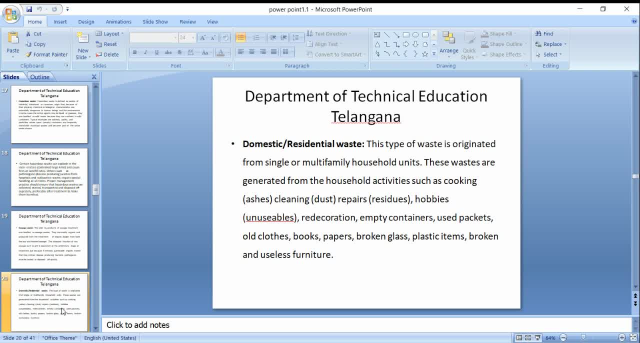 residential waste. this type of waste is originated one single or multifamily households. these waste are generated from the households activities such as cooking. so in the residuals also we have seen The paste which are coming from the ash and the garbage. So the garbage also one part of this. one domestic, So from the domestic only those done. So all ash cleaning, cleaning, dust repairs, spooking, all will come from. This is from. also the cancer has a residual. 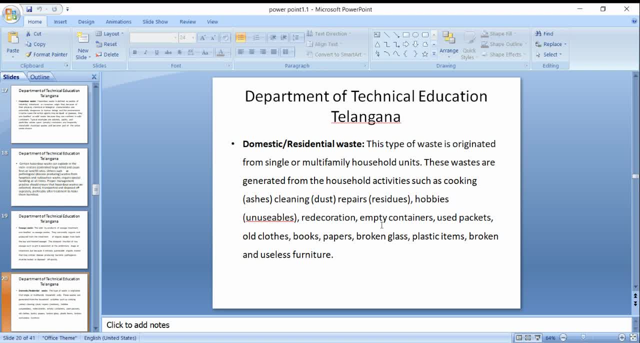 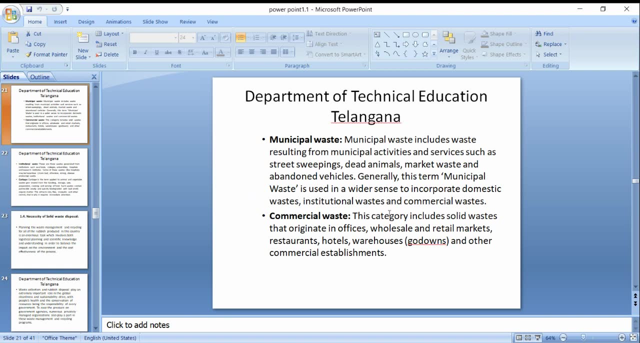 Empty containers, used packets, old clothes, books, all broken glasses. All this will come from the residential items. So next comes to municipality waste. So municipal also includes some resulting from the municipal activities and services, such as the street sweepings, dead animals, market waste. 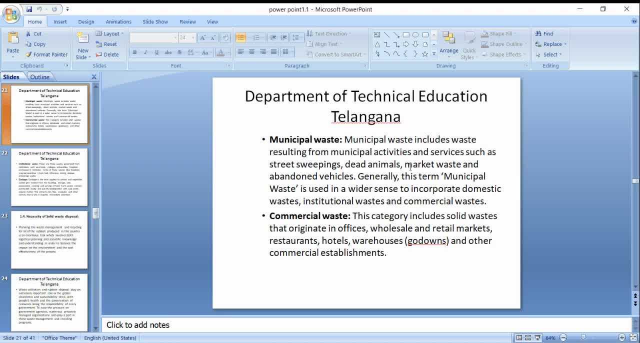 So in the market Ash also, we have different vegetables are there. So in the market waste and abandoned vehicles which are not useful, Those also. generally the term municipal waste is used for the wider sense in cooperative domestic waste institution. So municipality waste means nothing but which are not in use vehicles and dead animals. 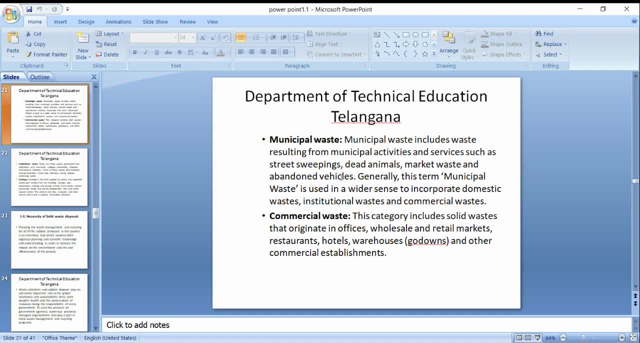 Those will be collected by the municipality, Municipal waste and those are considered the animals which are died on the street and the waste which was at the market, a market yard and markets. So those are considered as a municipal waste, Commercial waste, This categorized. 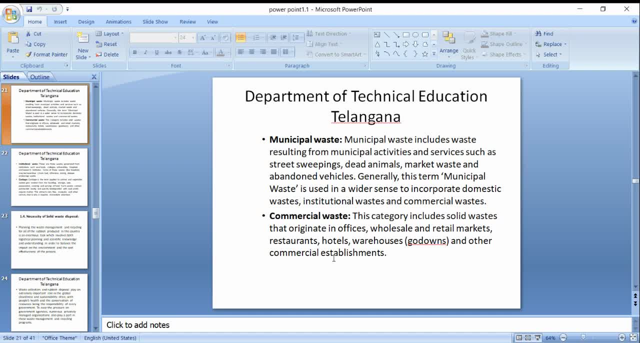 This categorized includes all solid waste that originates from the office, wholesale and retail market. So domestic waste is us that exist in workplaces, retail areas, restaurants, hotels. Regular layer is, for its garbageнюal, commercial Seungthe. procedures and orders can not be implemented. 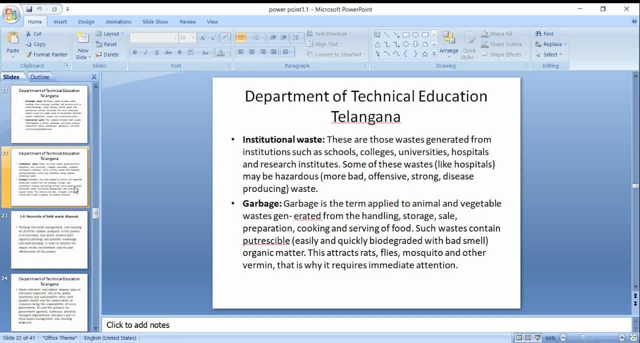 With the surrounding area. So all of what can be decided are left. Internal waste- This is An international Brother. Natural waste- When is Tourists? So the water through some papers and we will have some wasted covers. so, and mostly the 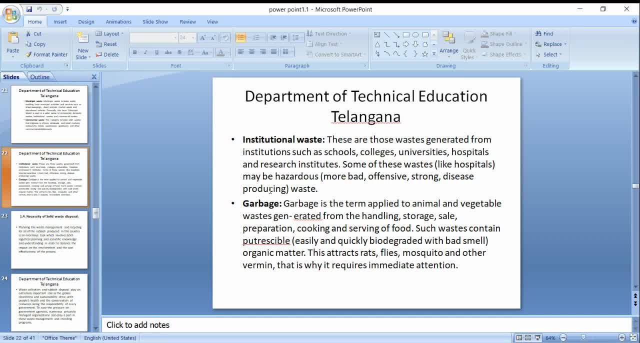 talk test you can say: and just okay, and research institution mentioned in the hospitals and the research Institute, so hospitals, we will get hazardous, more bad fences, strong disease producer. so generally from the hospitals we will get more hazardous waste. no more danger waste, waste. sanitation curtains are syringe, are you? 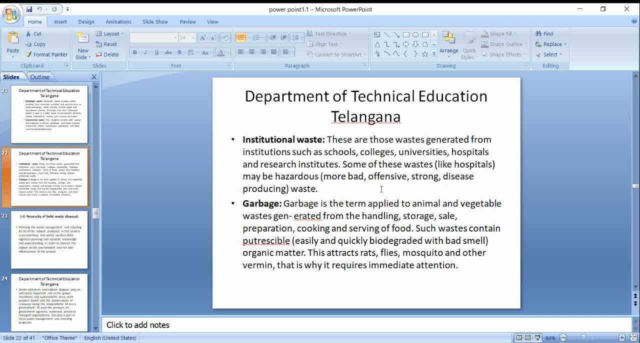 you. lot of waste will become bad. you can say injections of a bad syringes, so they will. all those are considered as a hospital hospitality waste, waste, garbage, garbage is nothing but applied to the animal at the visit. vegetable based- based which is produced from the animals and the vegetables of insurance. a. 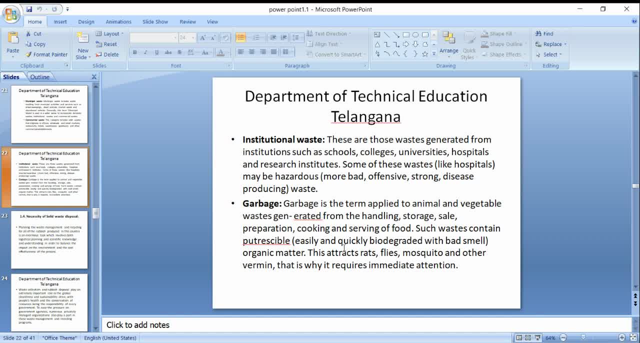 garbage so that you will be storage, sale, preparation for the cooking and so the garbage tables, and then in this to pay, well, stored and it will be sold. so this this can be, so that it can be put to participate and it will create and it easily decomposed okay. 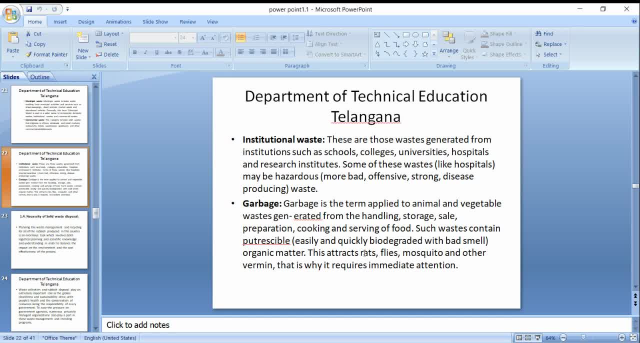 easily decomposed organic matter, so this attracts rats, flies and mosquitoes. so you immediately decompose the organic matter, so this attracts rats, flies and mosquitoes, so immediately. it should also repeat: it should not be placed directly, should also store it someplace and collected and we have to say we can sell those and we can do the vermicost, vermicomposting. 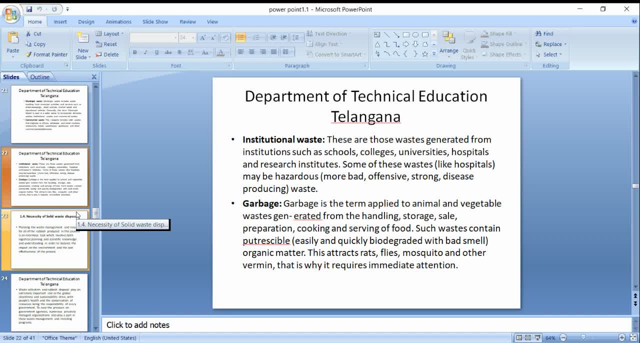 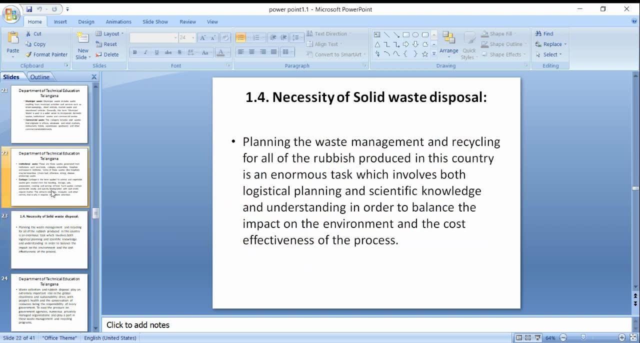 by all those. if it is a animal- cow dung is there we can use for the biogas productions like that- the recycling should be there, not it should be wasted like that. so about all these classifications? so next comes to necessity of the solid waste. so why solid waste? so till now we have seen the solid introduction to the solid waste. 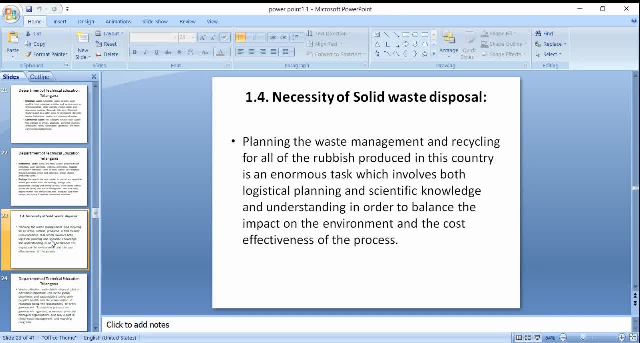 and comes to classifications. so in solid waste introduction is nothing, but we have planning. proper planning should be there for the segregation and the collection and further transportation, so that will be looked after by the municipalities. different local bodies are there in different states, so those will be looked after that once for that. 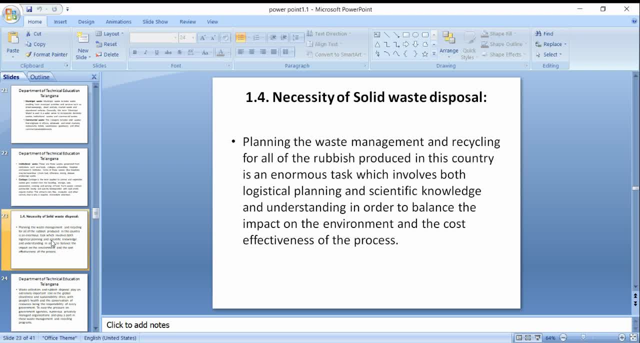 purpose. we are studying about the solid waste management after come. after that, one class patients are there, so different class of patients are there, so different ways, have divided into different, uh, categorized so that they will not get mixed into one. then and it is consider into one, then it will have some physical and chemical changes will be occurring so that 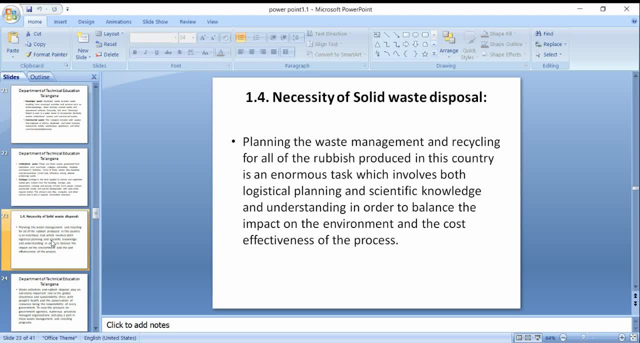 way they should be segregated. so for that purpose we have classified. next comes to necessity what, why it is required. so it is disposal. so planning the solid waste management and recycling of all rubbish produced in the country is an anomalous task which involves both planning and management. 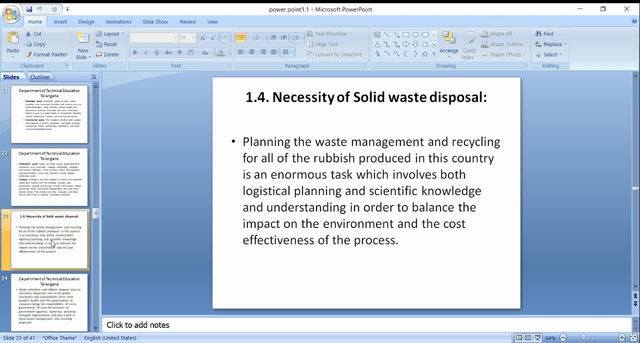 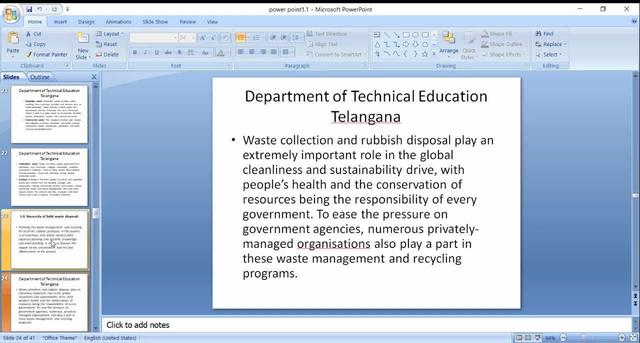 scientific knowledge. so planning the waste management is present and recycling is also important. so in the country it is becomes a big task. so in order to balance the impact of the environment, the cost effectiveness also should be considered. so it should be controlled away and also cost should be considered. so waste collection and rubbish disposal play an extremely important 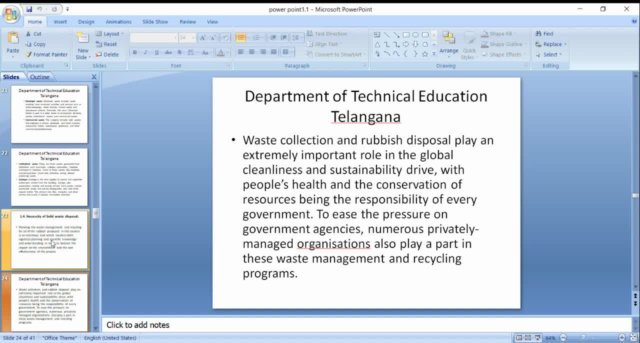 role in the global cleanliness and sustainability drive, with the people's health and the conservations of resources. so it's a response. so the task was taken by the government. so the collection and the disposal- this is a main thing- so that the government should be balanced with the cost effectiveness in the controlled way. so is to ease the pressure on the government ages. 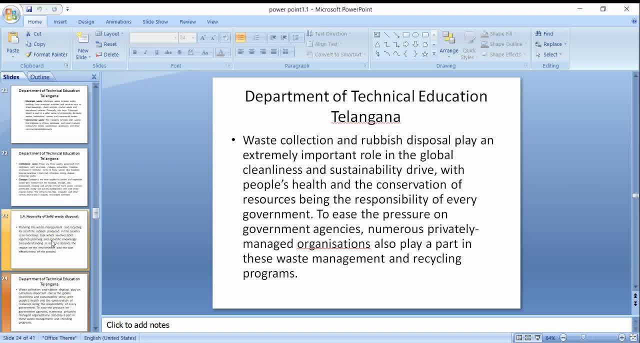 and So, and numerous privately managed organizations are came to play a part in this waste management. so some people will get: if you Thrown, if we, if you thrown out our keep in the house with unwanted plastic, Broken waste, will be they broken plastic waste, broken chairs, Broken glass, like that. that, if, if we stored like that, some people will take. 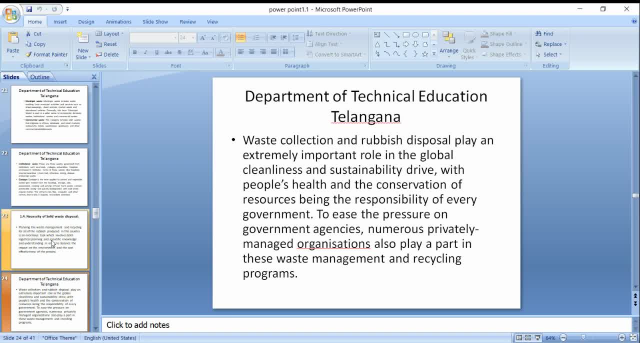 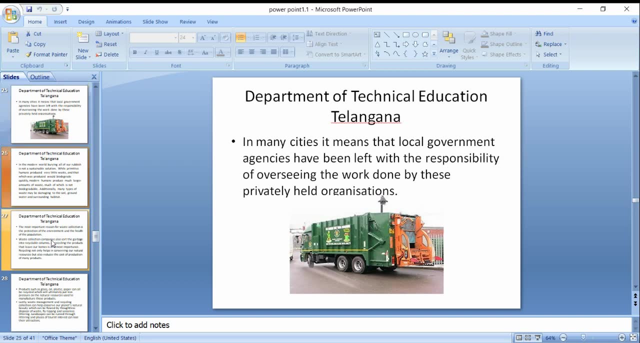 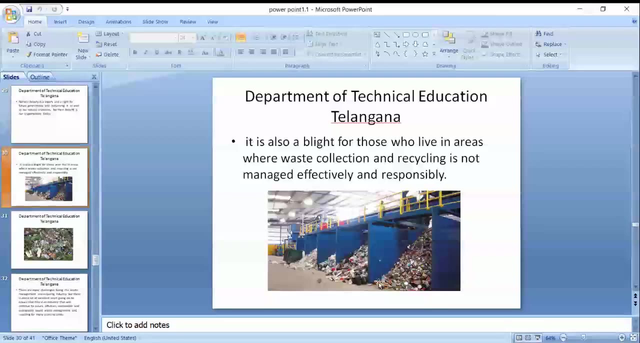 those things able in the day. in can say, in the Municipalities only some people will gather those things and they will put it in the Recycling, so they will segregate and they will use it right here here. this Like this. so the waste will be taken and it will be segregated. glasses like this plastic will be, and 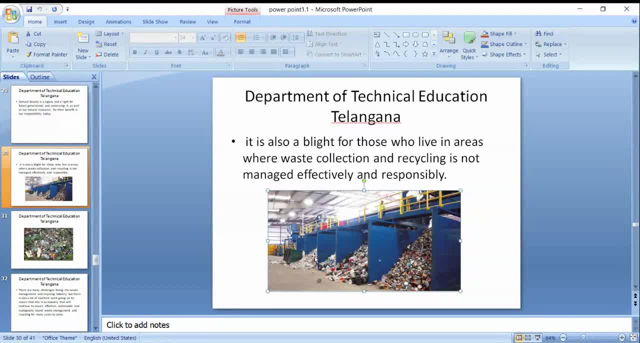 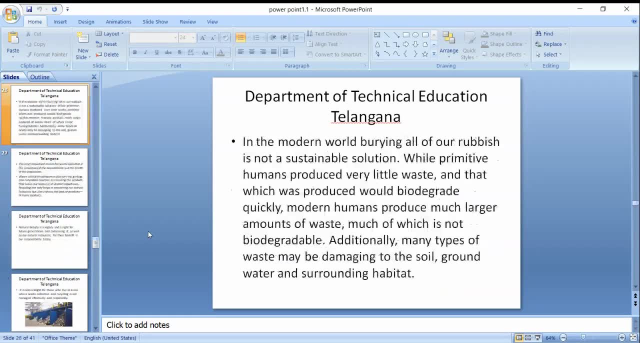 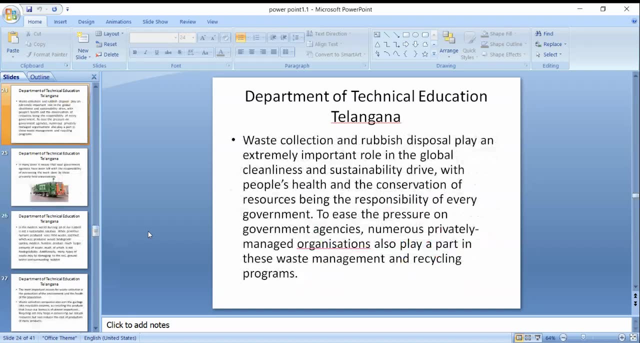 The paper and the ash and the concrete. like this, They will be segregated and they will dispose of some. further to, some private Organizations came to take all those that have became a part of this one map- waste management, So they will get Money at the same time. 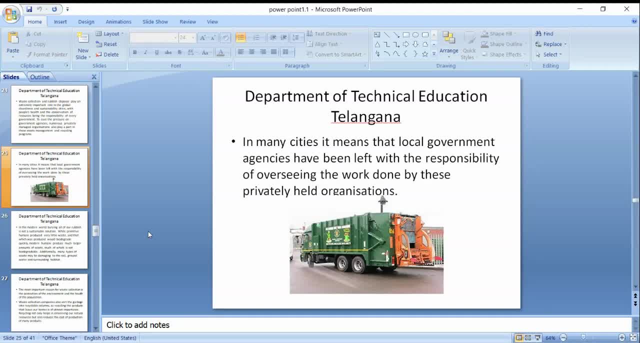 So in many cities it means that local government agencies have been left with the responsibility of overseeing the work done by these privately. so in many cities This is transportation like this We have to do the local government. It is not exposed and it will not create any type of pollution here. 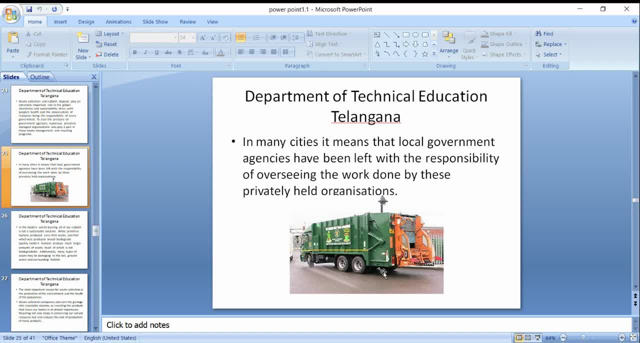 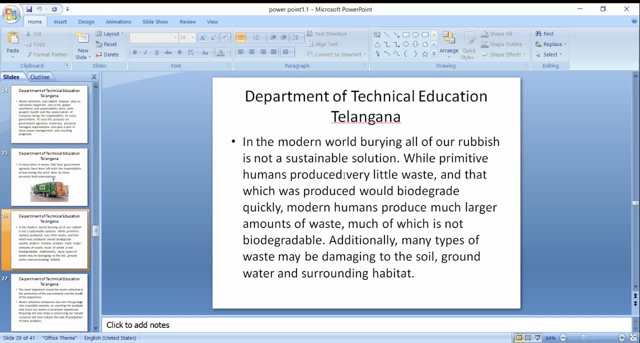 to the surroundings also, So it should be closed. so in the modern cities, burying and of all rubbish is not a sustainable solution. so in the previous, what the they are used to do, all the waste will be buried at one place and that will be that will be dumped at the low lying areas that create. now, afterwards, they created a soil, soil. 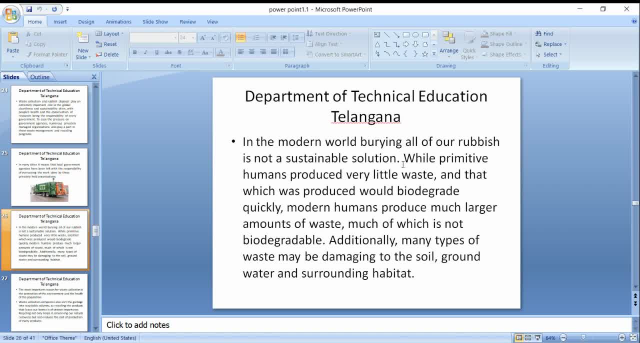 uh capacity. afterwards it created a soil problem. so for that, at present we are not burying the rubbish, so um, while permitting humans produce a very little base they, so they are used to little waste. only nowadays they are using a number of n number of, so we are producing. 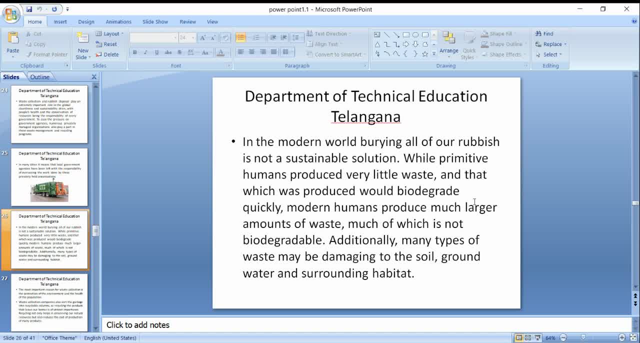 more waste compared to the earlier days. so modern humans produce much larger amounts of waste, much of which is not biodegradable. for example, plastic not is the biodegradable, and the glass is also non-biodegradable. like that, we are using many things which are not biodegradable, so for that we are damaging the soil, groundwater also. so 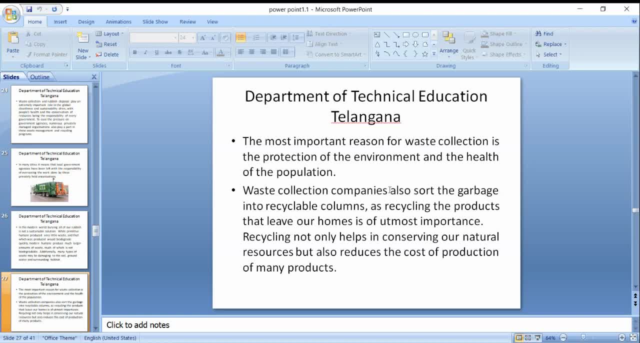 the most important reason for waste collection to protect the environment. so for that the the solid waste have came so main is to protect the environment. so how to collect that one and how to dispose is the major target to them. so waste collection companies also sorted the garbage into. 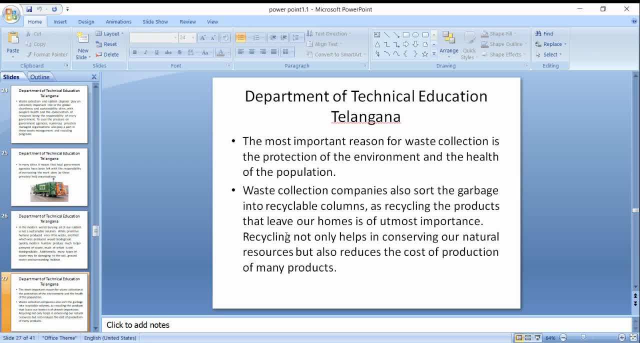 recyclable and the products that leave our homes is at most importance. so recycling not only helps in conserving our natural resources, but also to preserve our natural resources, our also reduce the cost of production of many products. for example, if we use the plastic, which is recyclable, that can be used and number of so by taking the 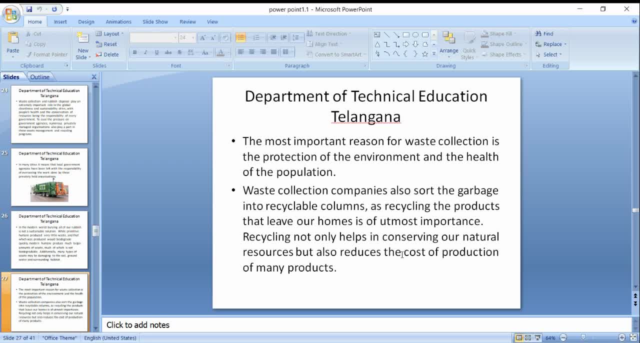 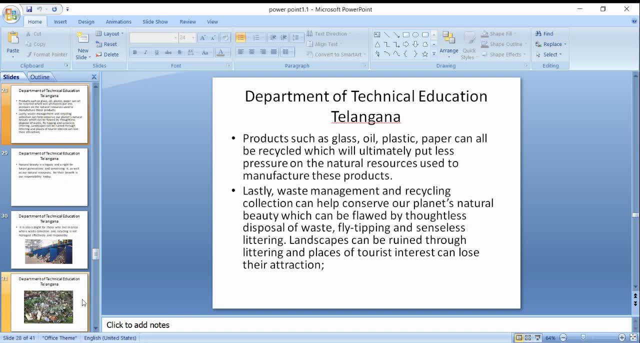 waste only. we are getting the other plastic material so like that, with reducing the protector cost also. so oil, plastic, paper and recycle, which will ultimately put less pressure on the natural resources used to manufacture. lastly, waste management and recycling collections can help conserve a planet's natural beauty and senseless littering goes. littering is nothing, but you can. 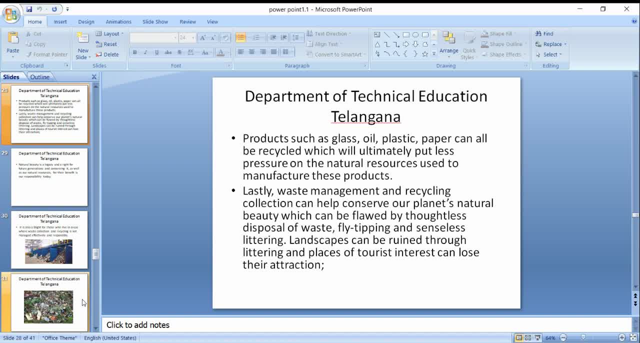 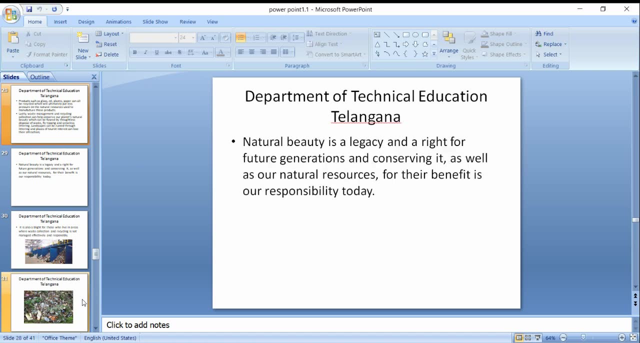 save them from waste. some water will be disposed, so the water will also pollute the surroundings. so so littering is nothing but so pollute the surroundings. so so littering is nothing but so. but the base which is coming from the plants, so that can also come less so. 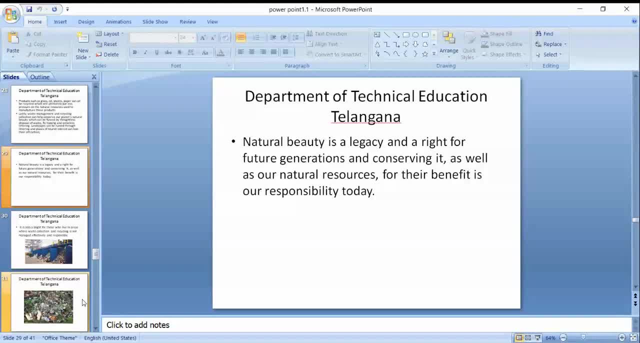 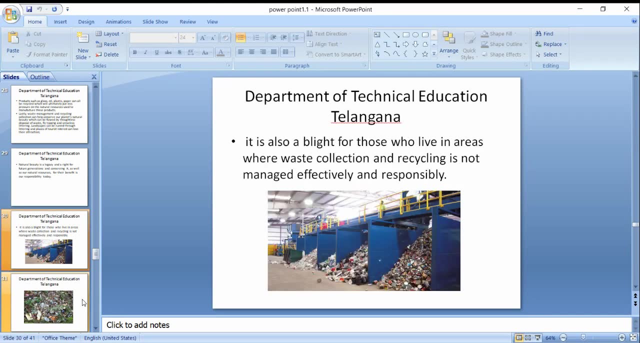 it's a natural beauty also. if we control the waste management, then future generation also have good future well, and they will also enjoy the natural resources. by doing present in fit of so like this, we will be segregating so who live in areas where waste collection and recycling is not managed. 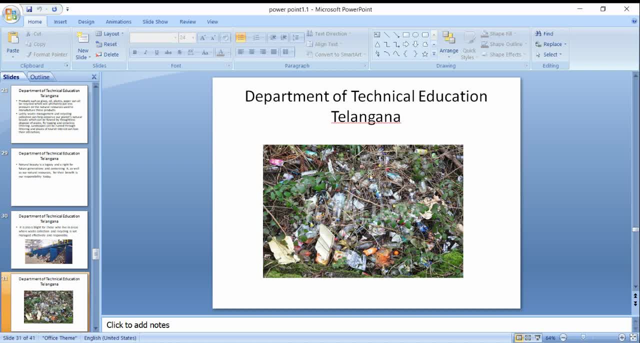 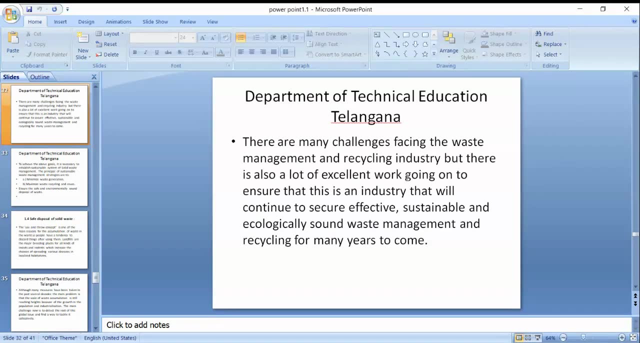 effectively and responsibly. so like if we dump like this, they will all these get like this here, rather waste, all are dumped like this, so it will pollute the surroundings. so there are many challenges facing the waste management and recycling but there is a lot of excellent work going on to ensure that. 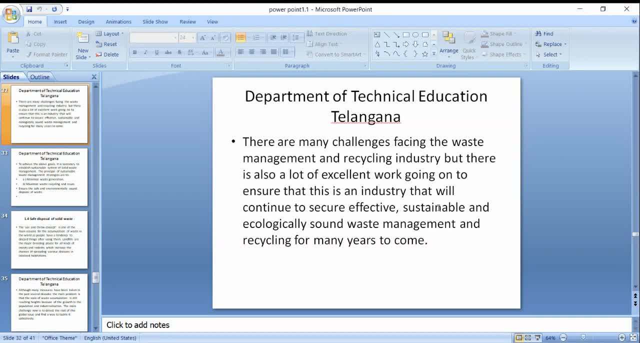 the waste is stored properly. so we are keeping a kind of physical and social. so we are keeping a kind of physical and social in this way, so we are keeping a kind of physical and social industry and that will continue to secure the effective and sustainable and ecological sound. 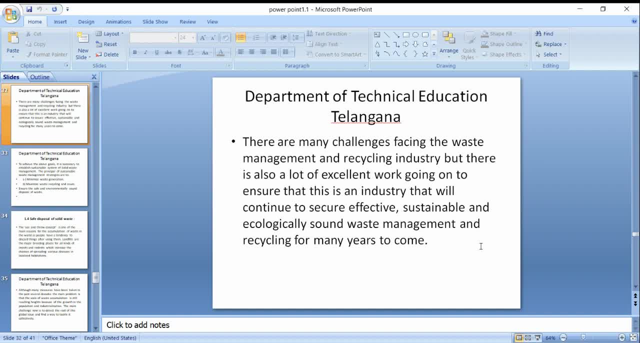 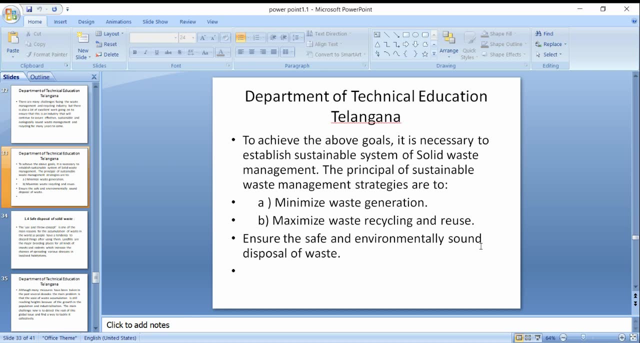 waste, so recycling for many years to come. so this is the nowadays. they are getting a facing a task- management- to them. so to achieve the above goals, it is necessary to establish a sustainable system of solid waste management. uh, the principle of male sustainability is nothing but to minimize the waste generation and maximize the waste recycling and reuse. 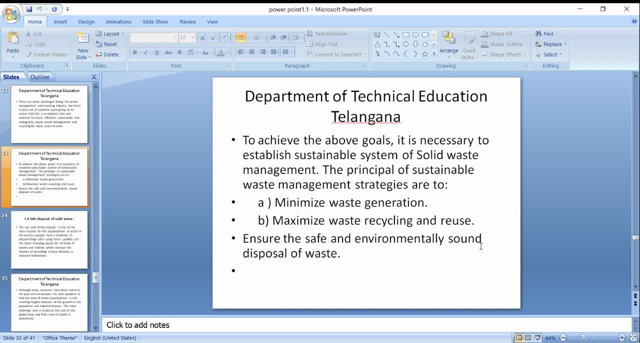 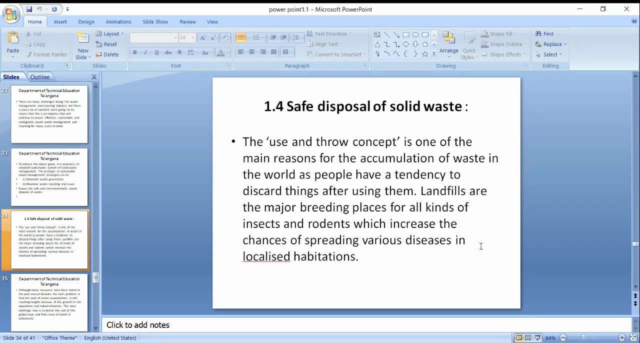 so first, base should be minimized and it should be recycled. then only the environment is in the safe zone. ensure safe and environmental. so so next comes to here. we have studied, report the three subtopics: first comes to interaction, x comes to classification and third comes to the need. next, last, whom comes to? 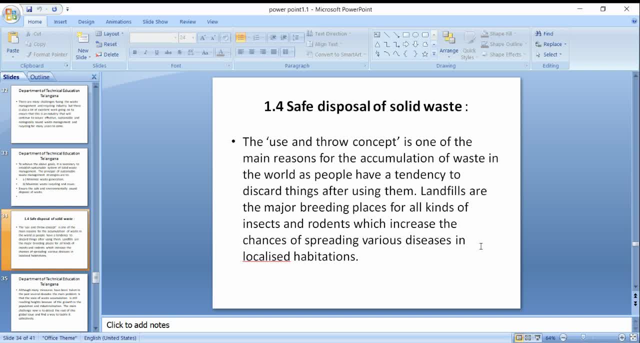 safe disposal of the solid waste. so the use and throw concept is one of the main reasons for the accumulation of the waste. so we generally what the things we are using if it is not used means. we will think about the throwing of such things. so use and throw is the 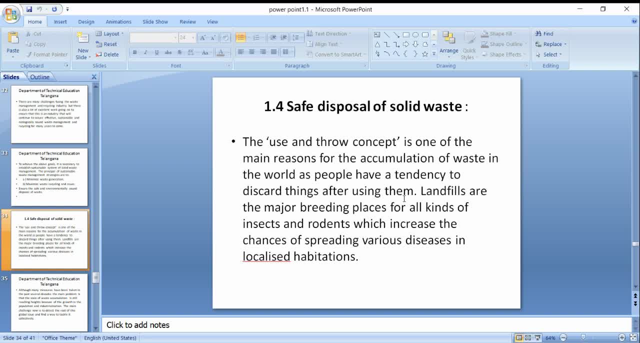 concept. but the safe disposal is there and so accumulate over the world has. people have to tendency to discard the things after using them, so landfills are the major breeding places for all kinds of insects and rodents, which increase the chances of spreading of various diseases. so if you thrown the paste in the open dump yards, it has creating the major breeding. 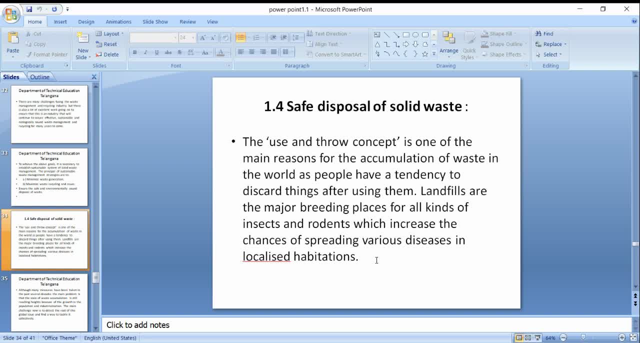 breeding places that will create the spreading of our diseases. so lots of nowadays we are getting the dengue typhoid. are all these if? if we go for the cholera, that was contaminated with the water, so the waste which was dumped on the open air that has polluted the groundwater also. so, like that, 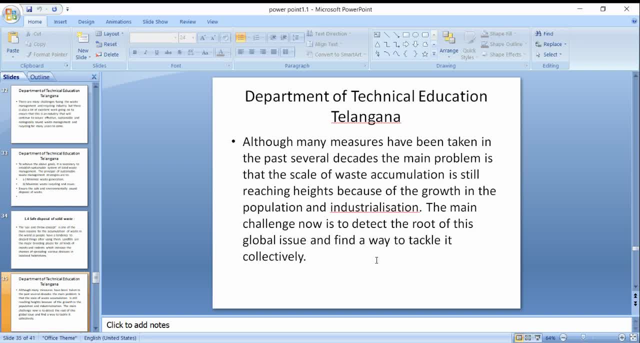 the different types of the pollutions are created. although many measures have been taken in the past several decades, the main problem is to scale of waste accumulation. so it's a reaches heights because of the growth in the population and the industrialization. so several decades we have trying to reduce the ways, but it is reaching. 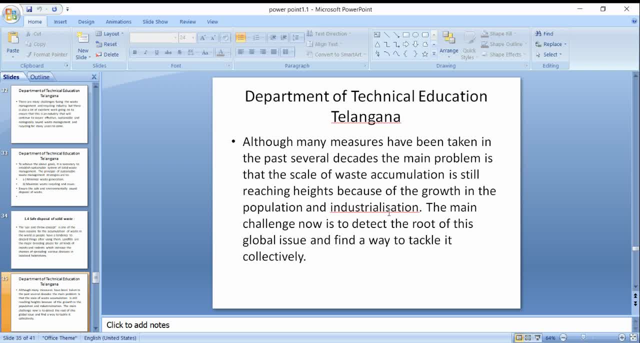 the better values than the growth. we are trying to reduce the ways, but it is reaching the better values than the growth, but it is reaching the better values than the growth. so, more by more, the growth is increasing. the produced invitation of it is increasing because of population iscombasing at the same time. 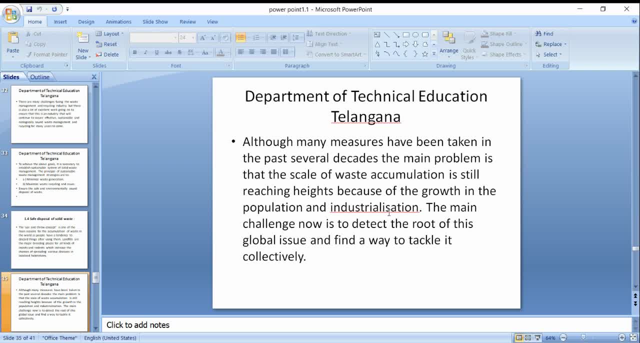 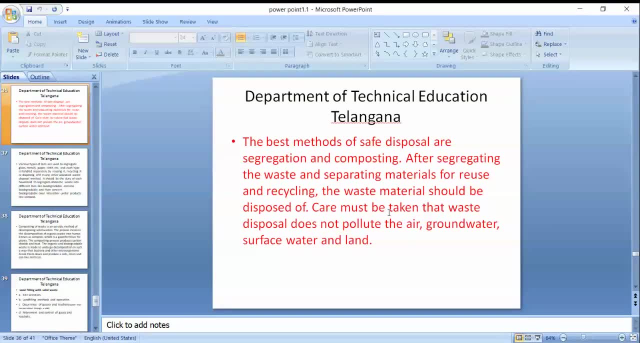 now the information also. it is it. so both are ocean lion. its position is increasing, so both are getting increased, more targeted growth. so that's why, with its picking and a challenge global issue how to resolve the things. so the best method of safe disposaltions are named compostable food and food composting, etc. lead in the best method, the best method for How to stopped compensation people are supposed to serve. who cites bio Bea Jai. they're acid Aie tot Southwest of sad hits. which will stop videos from Healthist. just know what another source probed about either getting together myaret media support and how to 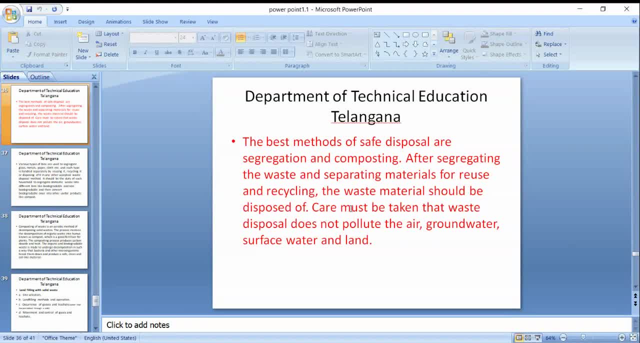 So after segregating, it should be either recyclable or composting. So after segregating the waste and separating materials for reuse and recycling- So if it is reuse we have to think it is not- then we have to compost the materials. So the waste material should be disposed of and care should be taken. 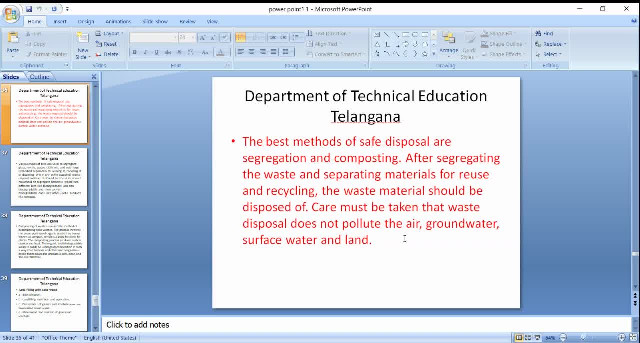 Then the does not pollute the area, groundwater, surface and water. So when we are not using the waste, the waste should be segregated. First of all, we have to segregate it, Okay, after getting collected and it should be disposed at one place. after disposing, it should be segregated. 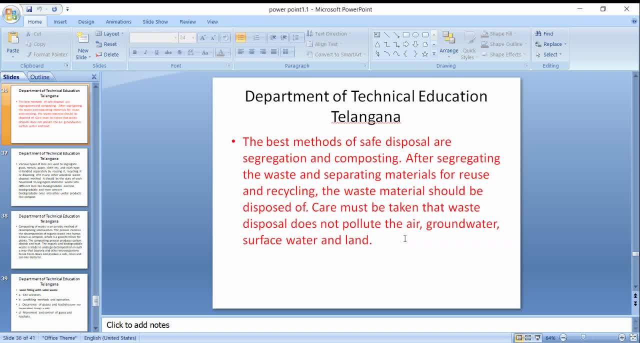 If, after segregation, We have to think about the composting, Composting comes when, after separating the reuse and the recyclable things, If it is reuse and recyclable things are separated, then other waste, just like food waste, Okay, those can be composited. 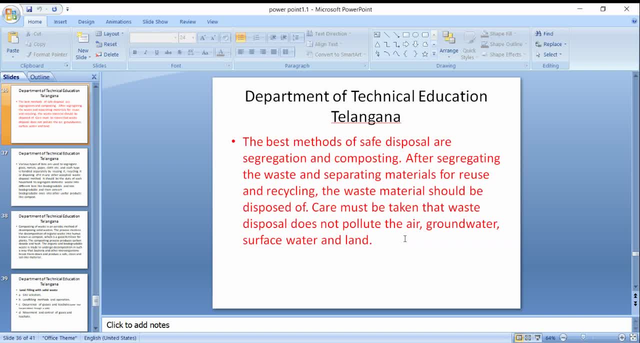 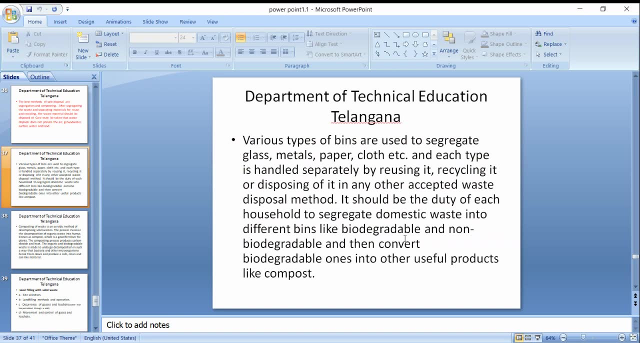 So the composite animal waste or food waste, those can be composited, So by that we can reduce the air Pollution of the air in the ground water. So various types of segregating: glass, metals, paper, cloth, and each type is handed separately by reusing it. 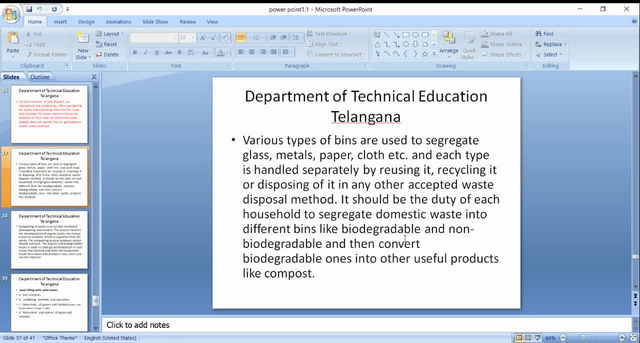 So those are reused, recycling, it are disposing of it any other accepted waste disposal. So it should be taken permission and it should be reused, Recycling, Recycling, Recycling. It should be the duty of each household to segregate domestic waste into different bins. 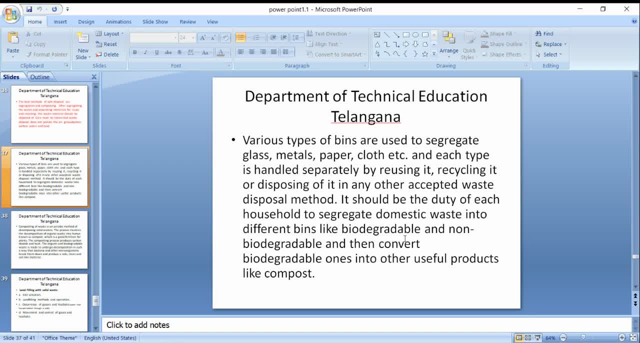 So dry waste and the wet waste, like that, we have to separate it and that waste is thrown in the different dust bins, also Like that in the house itself. if we maintain like that, we can segregate from the bottom house And you can say biodegradable. 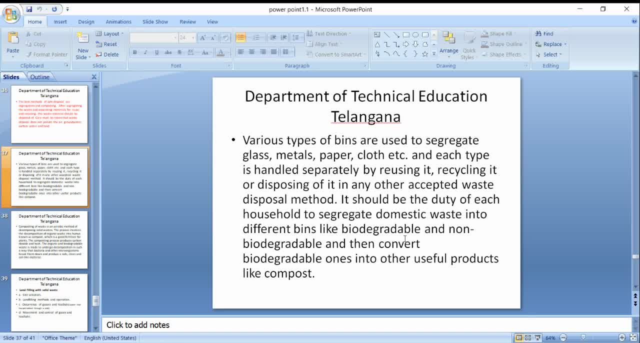 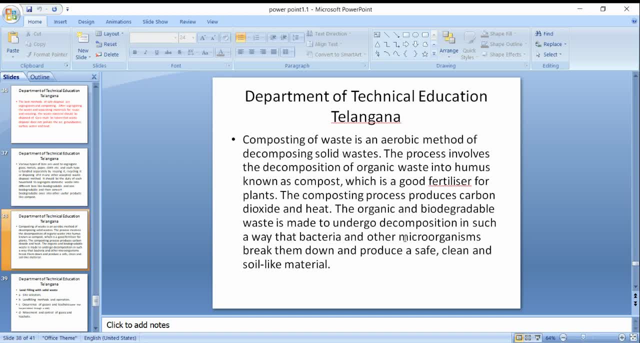 Biodegradable that can convert into useful products like compost, like that we can say. next, compositing of the waste is an. compositing is nothing but the aerobic method. anaerobic method and aerobic methods: both are. the aerobic method is nothing but the presence of the oxygen at the anaerobic method is the absence of the oxygen. 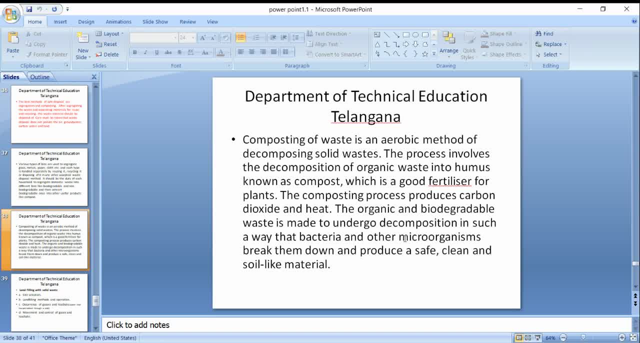 So it is. It is. It is Exposed to the sun. So aerobic method of decomposing of the solid waste. the process involves the decomposition of the organic matter into humus. So the if it forms a humus, that will be useful for the plants, which is good fertilizers for the plants. the compositing process produce the carbon dioxide and the heat. 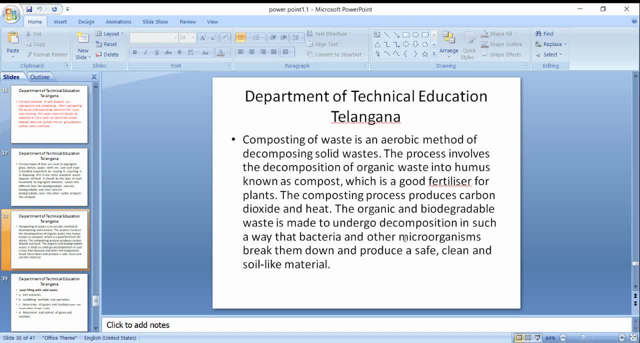 So when it is changing the The organic organic waste so into into organic waste, there they produce the CO2 and the heat, so the organic and the biodegradable waste is made to undergo the decomposition in such a way that bacteria and other micro organizations break them down and produce a safe, clean, and so in this we can use the two methods are there. 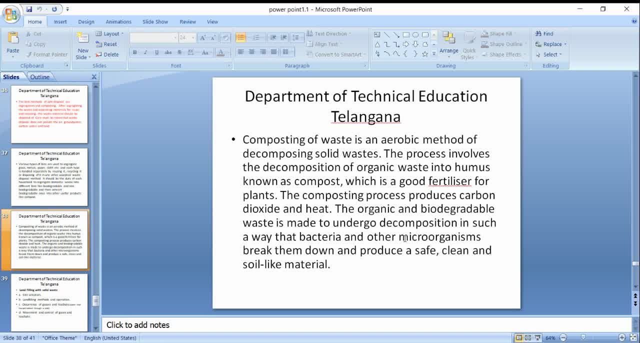 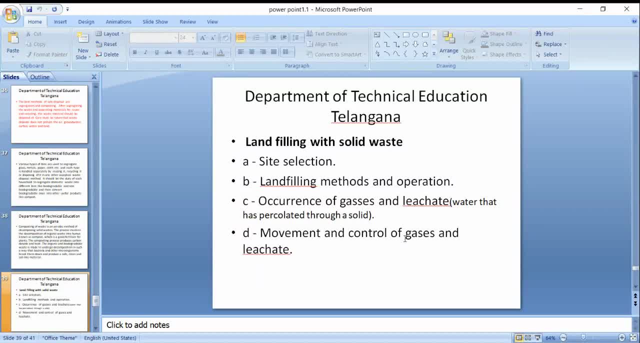 So we can use the two methods. are there- Bangalore, Bangalore- indoor method is generally preferable. So we can use the two methods. are there, Bangalore, Bangalore indoor method is generally preferable. However, I need to mention then this land fill in medicine. However I need to mention, then this land fill in medicine. 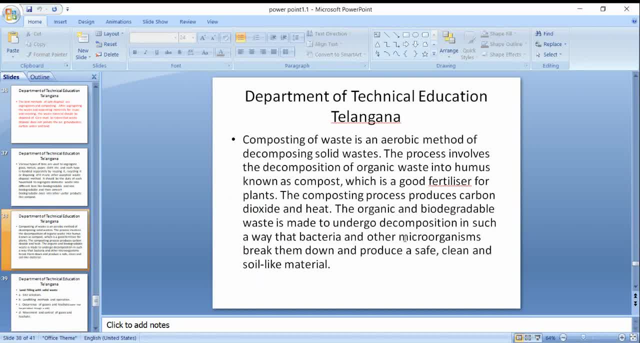 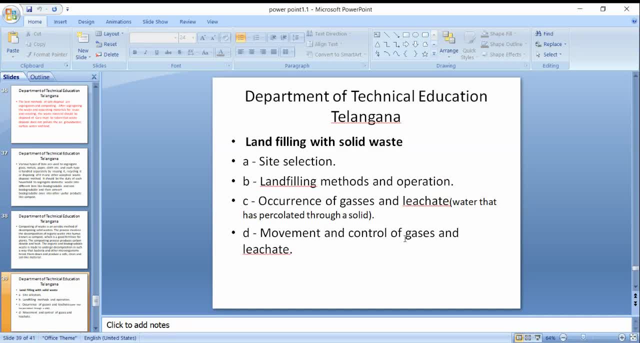 So how to dispose so in the disposal? So how to dispose so in the disposal gl when filling metas. So what do we do now? here we have to choose the site, всё, And then we have to fill in the distanceuss, And then we have to choose the site. 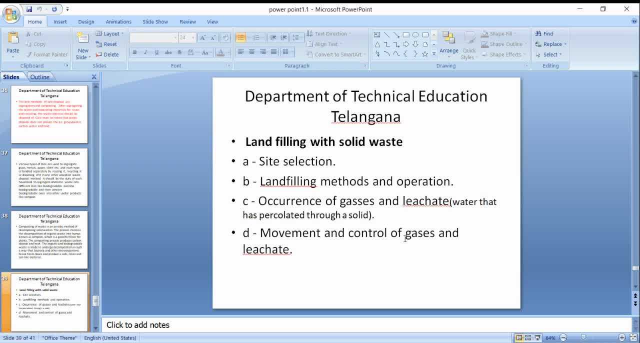 Now Facebook is open to theī, so when filed a multiple second or a над is the gases in that one. so glasses in the Richard. Richard is nothing but the solid. if we go so, from the solid getting composed, the water get percolated to that one, and so the you can say bad water. it is coming so moment and the 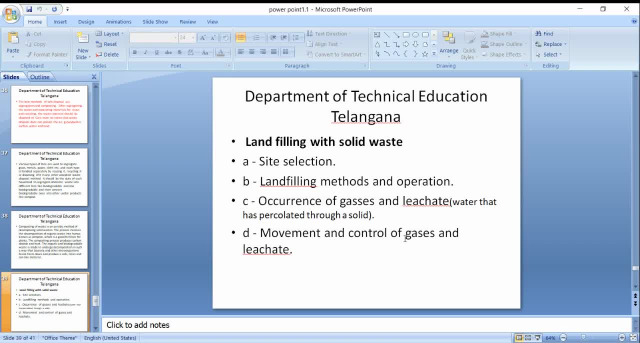 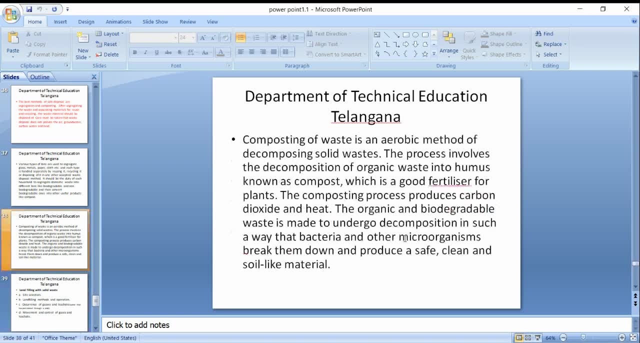 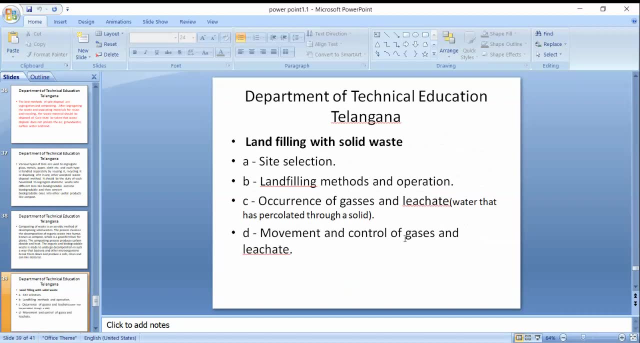 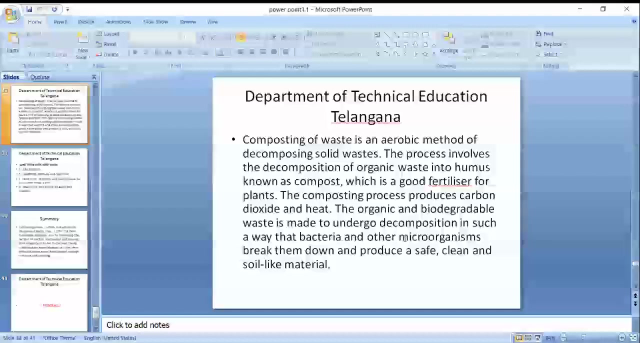 control of the gas is also there. so in the in this, we have seen only the land feeling better when they insulations. and the burning- burning- all different feathers are there in the solid waste disposers in can next coming up chapters, it is they so. so in this, we have studied a photo. 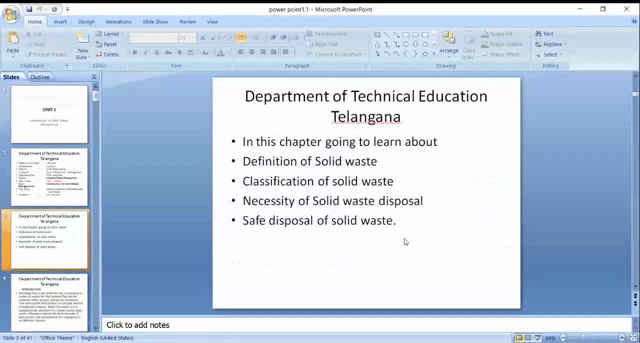 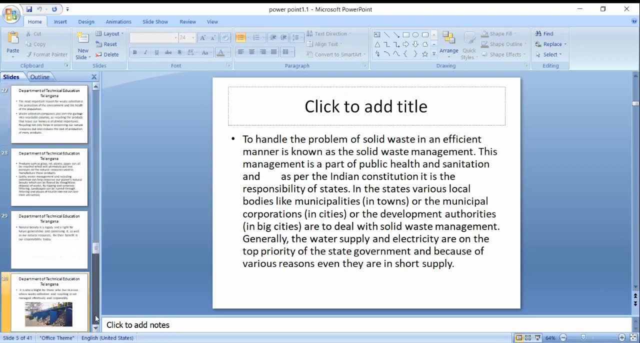 covered definitions of the solid waste. we have covered the classification of the solid waste and the definition of the solid waste. we have covered the classification of the solid waste and we have covered the necessity of the solid waste and also safe disposers. so these are the different types. we have us covered here.